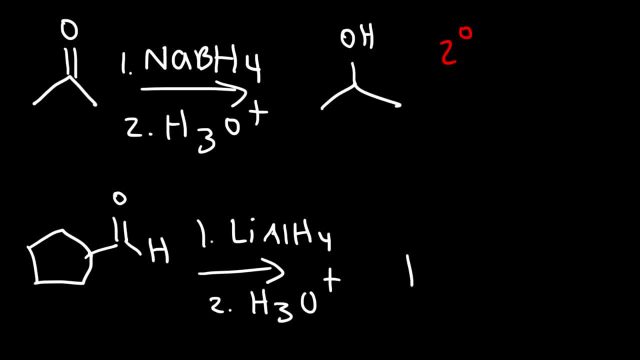 The end result will still be the same, And that is, the carbonyl group will be reduced to an alcohol. So in this case we have a primary alcohol. Now let's go over the mechanism of the first reaction. So here we have a ketone and we're going to react it with sodium borohydride. 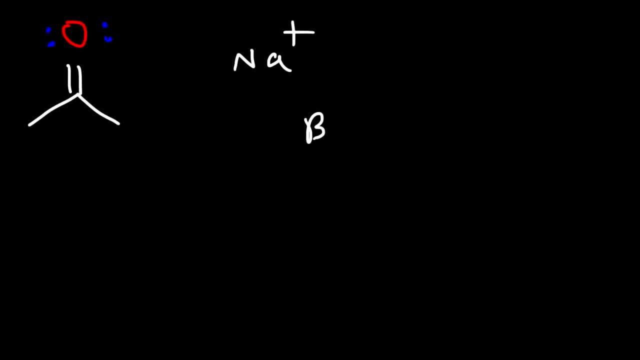 So the sodium ion has a positive charge and boron has a negative formal charge because it's attached to four hydrogen atoms And hydrogen is more electronegative than boron. So if you focus on the boron atom, you're going to get a ketone, And if you react it with sodium borohydride, 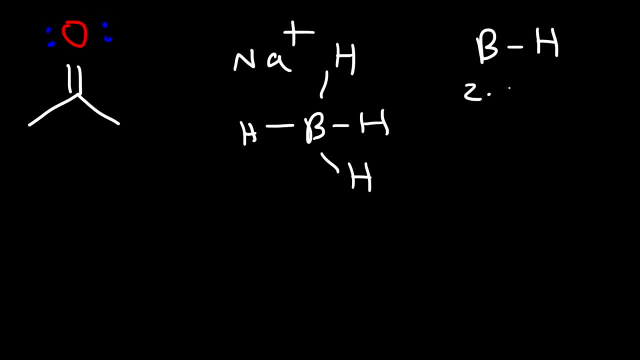 boron has an electronegativity value of approximately 2.0.. And for hydrogen it's 2.1. So therefore, hydrogen is slightly more electronegative than boron. Therefore it has a partial negative charge. Now the carbon atom of the carbonyl group. 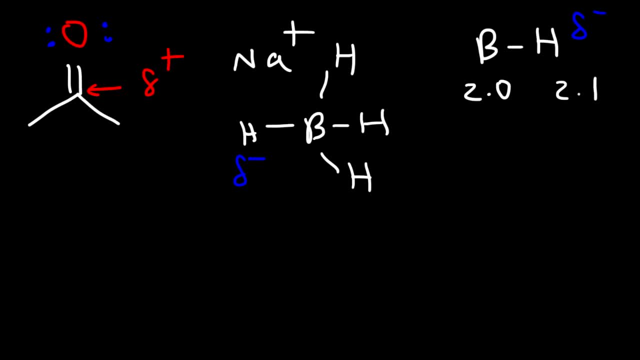 contains a partial positive charge, And so this hydride ion, or this hydrogen with a negative partial charge, is a charged, And so this hydrogen ion has a partial negative charge, And so this hydrogen ion is attracted to the carbonyl carbon, So it attacks it And this is going to give us. 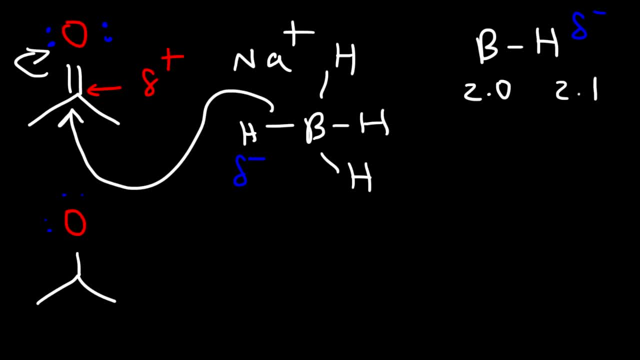 an alkoxide ion which has three lone pairs and a negative charge, And so far we added a hydrogen to the carbonyl carbon. Now, in the second step, we are going to react the alkoxide ion with H3O+. 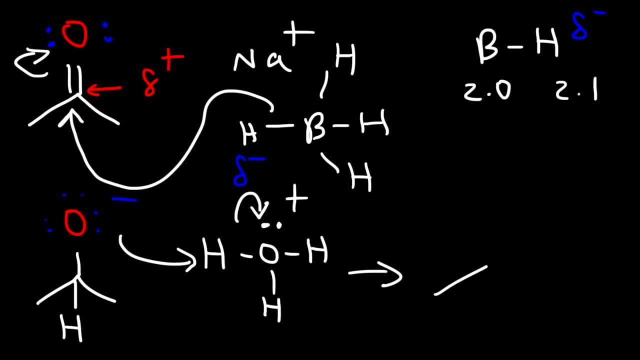 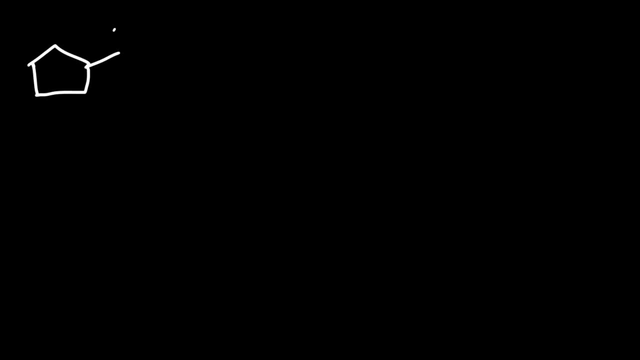 And so it's going to pick up a hydrogen, turn it into a secondary alcohol, And so that is the mechanism for this reaction. Now let's go over some other reactions. So here we have an ester, And let's react it with lithium, aluminum hydride, Sodium borohydride is not strong enough to reduce. 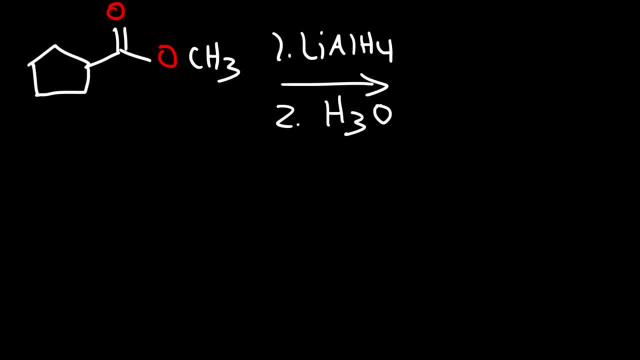 esters and carbosilic acids, But lithium aluminum hydride can reduce them all, So go ahead and predict the major problem. So let's say we have an ester which is a product for that reaction, As well as this one too. 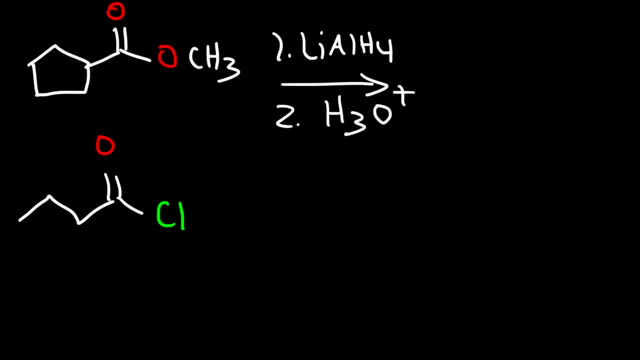 So let's say, if we have an acyl chloride And if we react it with sodium borohydride, with H3O+, Acyl chlorides are very reactive And so we can use a mild reducing agent like sodium borohydride. 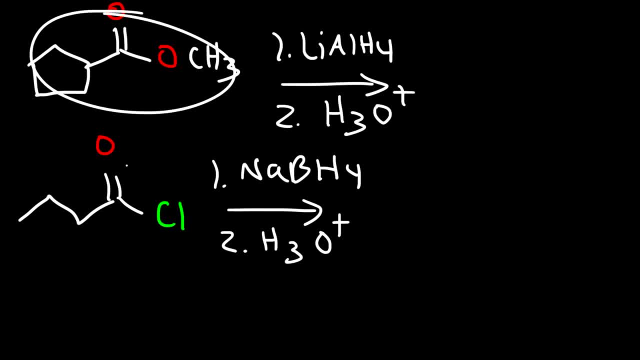 to reduce the acyl chloride. Esters are less reactive than acyl chlorides, So if you mix an ester with sodium borohydride, you're going to have a reaction that's very reactive, And so we're going to have a reaction that's very reactive. 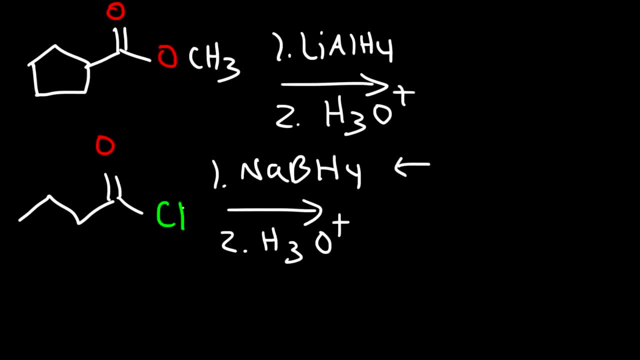 Nothing's going to happen. This is not strong enough to reduce an ester or a carboxylic acid. Now let's see what's going to happen if we take this acid chloride and react it with this reagent. So lithium, aluminum with three OR groups and a hydrogen followed by H3O+. 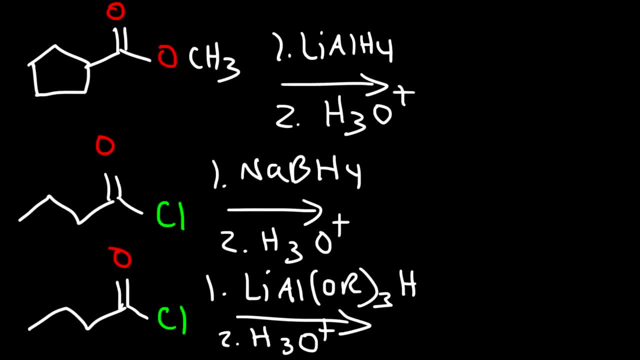 Now what you need to know is that lithium aluminum hydride will reduce the carbonyl group into an OH group or alcohol functional group. Now this bond will break, and so here we have our OH group. I'm going to put that in a different color. 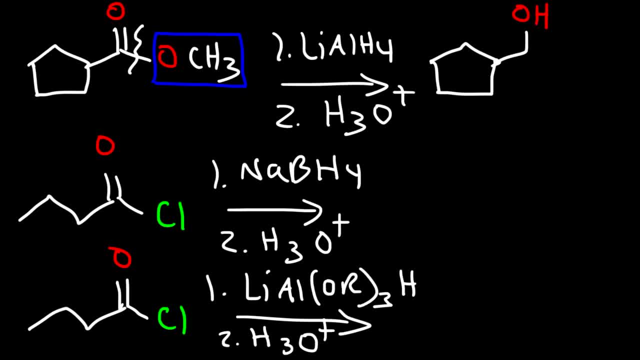 And this group here is basically the leaving group. It's going to pick up a hydrogen from the acidified solution, turn it into a hydrogen, and then it's going to take the hydrogen from the acidified solution and then it's going to take the hydrogen from the acidified solution. 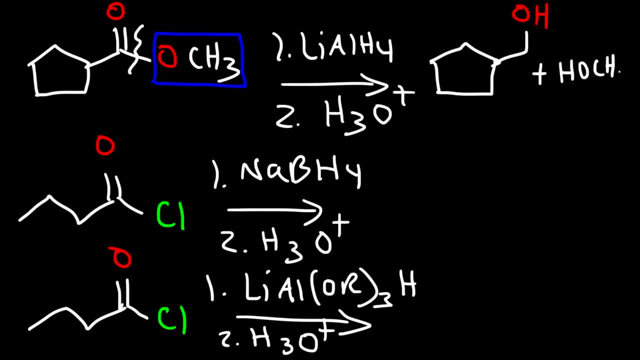 and then it's going to turn it into methyl alcohol. But the major product for this reaction will be the primary alcohol Now, sodium borohydride. when you react it with an acid chloride, it's going to turn into an alcohol as well. 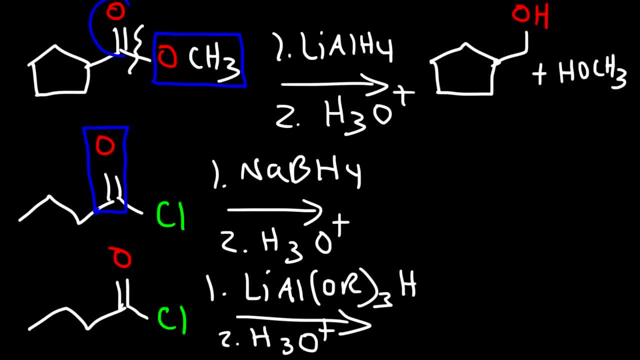 So this carbonyl group like this one will be reduced into an alcohol And the chloride ion will leave as a side product. Now if you see lithium aluminum hydride, but instead of having four hydrogens, it only has one. it can only reduce the acid chloride to. 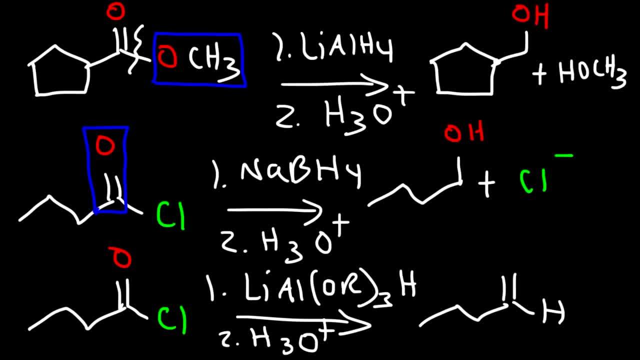 an aldehyde level. Another reagent that can do this is if you see a dye ball. sometimes you'll see an H attached to it. So if you see a dye ball, it can convert the acid chloride into an aldehyde as well. Now let's go over the mechanism for the 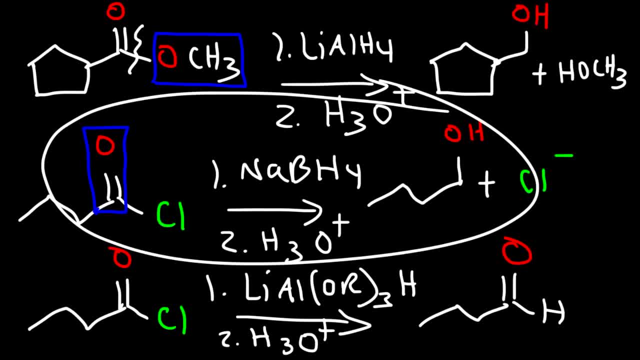 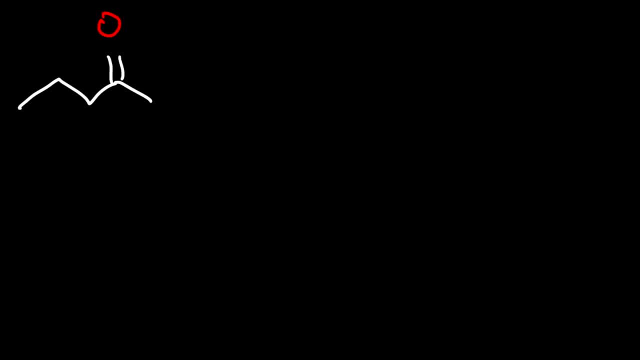 reduction of an acid chloride into an alcohol. So here is our acid chloride and we're going to react it with sodium borohydride. so let's not worry about the sodium ion, because it's a spectator ion in this reaction. the boron atom has a 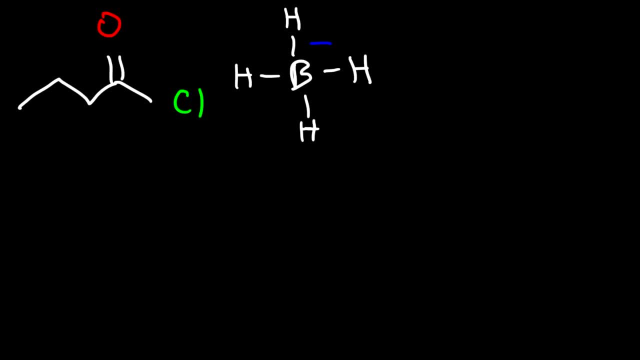 negative formal charge. but it has a positive partial charge because it's less electronegative than hydrogen. so don't let that confuse you. formal charge and partial charge are not the same thing. so the hydride ion, just like before, will attack the carbonyl carbon, causing a pi bond to break, and so we're. 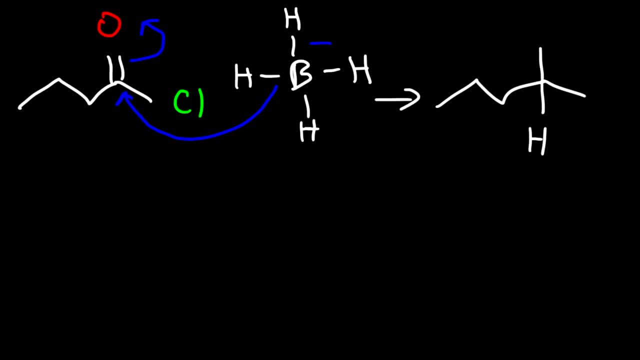 going to get this tetrahedral intermediate, and right now the oxygen atom has three lone pairs instead of two, and so this tetrahedral intermediate is unstable. so it collapses, reforming the pi bond, but expelling the chloride ion, since it's a good leaving group, and so by adding the first hydrogen we can go. 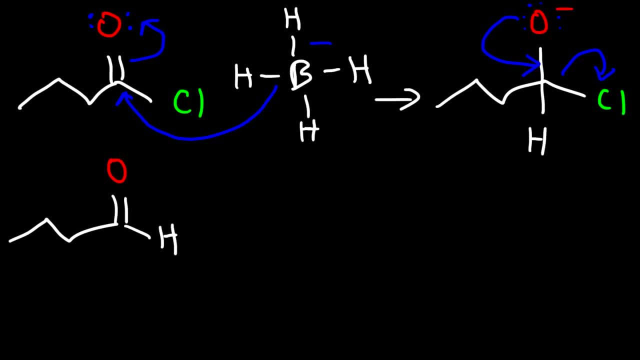 down from the acid chloride to the aldehyde level. but now sodium borohydride will react again with the aldehyde, so we're going to use a second borohydride ion. it's going to attack the carbonyl carbon, generating an alkoxide ion. 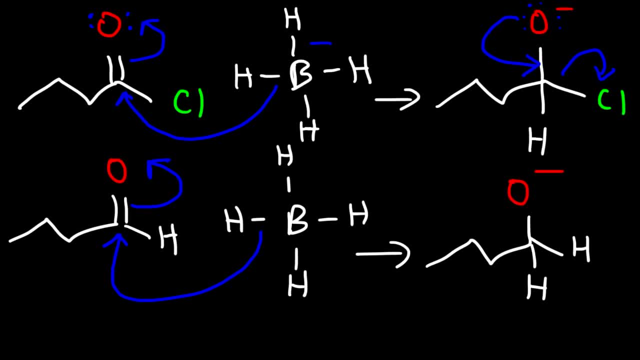 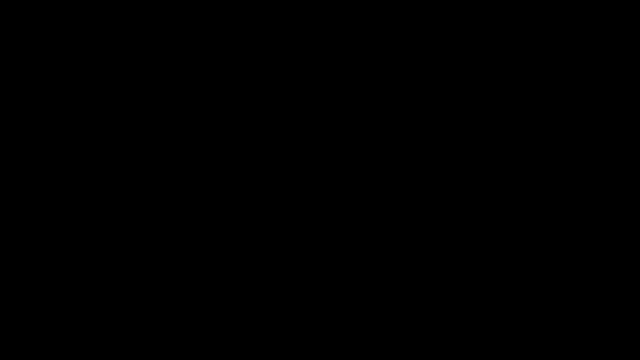 so far, we've added two hydride ions to the carbonyl carbon, and now the last step is reacting the alkoxide ion with h3o plus. so we need to acidify the solution, and so the oxygen with a negative charge is going to pick up a. 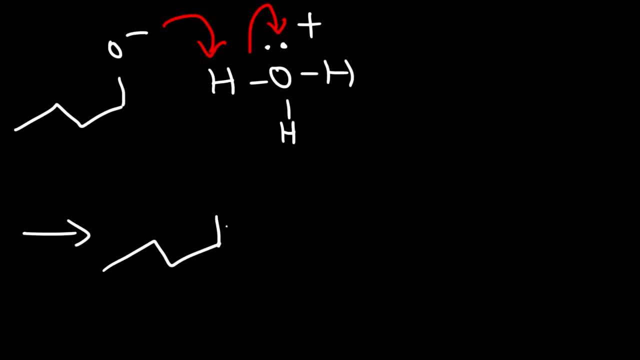 hydrogen, given us a primary oxygen, showed negative charges. given an imperfection, a hydrogenaste going to bouncy hahedron gives an oxygen hardening. pleased to scratch. So these are the two nucleophilic hydrogen. excuse me, these are the two nucleophilic. 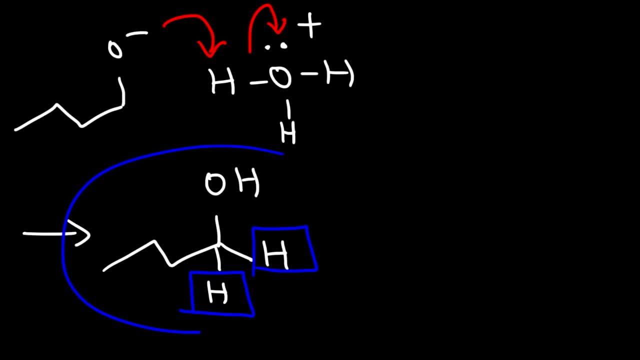 hydrogen atoms that we've added to the carbonyl carbon. And so whenever you react an acid chloride with sodium borohydride or even lithium, aluminum hydride, it's going to reduce the acid chloride all the way down to an alcohol. Now let's react the acid chloride with lithium, I mean. 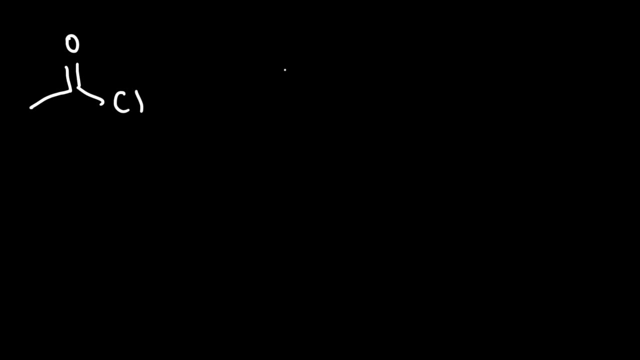 not just lithium, but lithium aluminum hydride, or at least a deactivated version of it. So instead of aluminum hydride, where it has four hydrogen atoms, we're going to use the one where it has like three OR groups. So this is lithium aluminum OR3 with a hydrogen, And so this is a deactivated reagent, Because 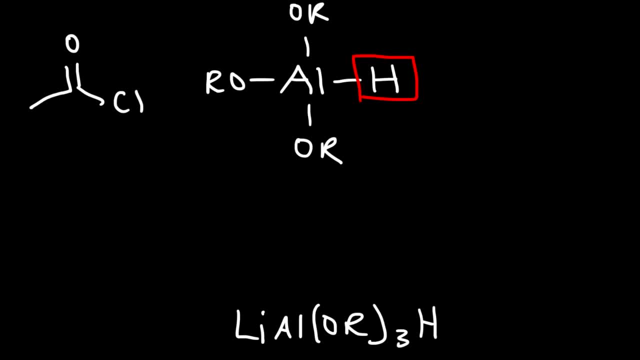 it only has one hydrogen. it's going to react with the acid chloride and stop it at the aldehyde level. so this hydrogen is going to attack the acid chloride and so we're going to get this tetrahedral intermediate and then it's going to kick out the chloride group. so the end result: 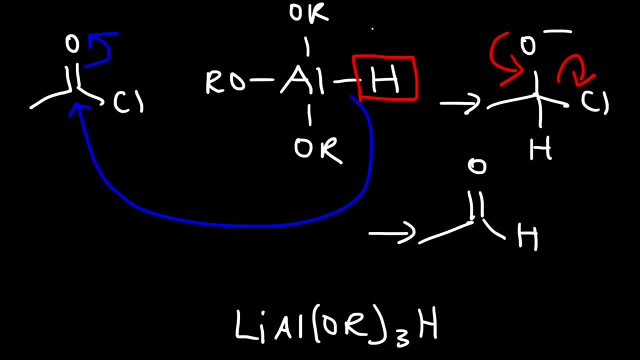 is the aldehyde. so if you, if you react one equivalent of this reagent with the acid chloride, the major product will be this: the aldehyde. it stops at this level because there isn't enough hydrogen atoms to reduce it all the way to an aldehyde. and so whenever you see this where there's three OR groups attached, 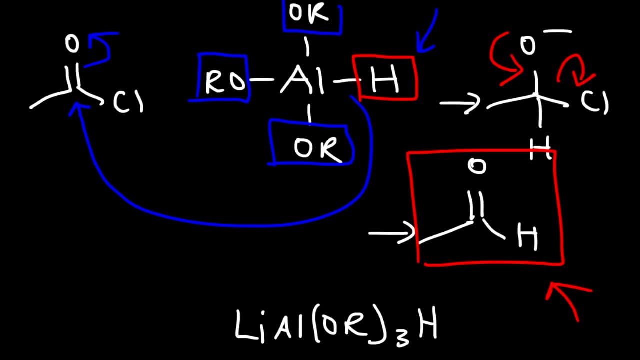 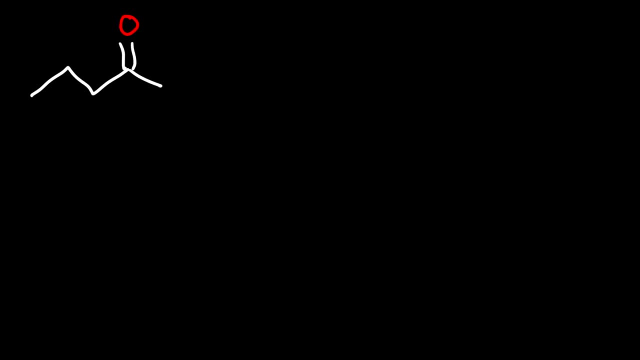 to the aluminum atom and only one, hydrogen. it's telling you to stop at the aldehyde level. so if you have a test, just look for the aldehyde functional group as your answer. now there's some other reactions that we need to review as well. what's going to? 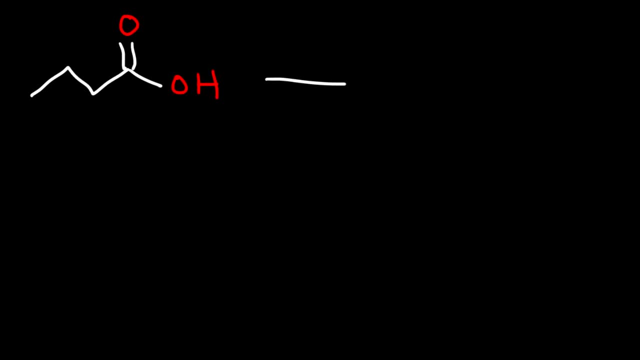 happen if we react a carboxylic acid with lithium aluminum hydrogen. I mean a hydrogen but lithium aluminum hydride, followed by HDO plus. so, just like the other reactions, the carbonyl group will be reduced to an alcohol and then this group is going to leave. it's going to pick up a hydrogen from the 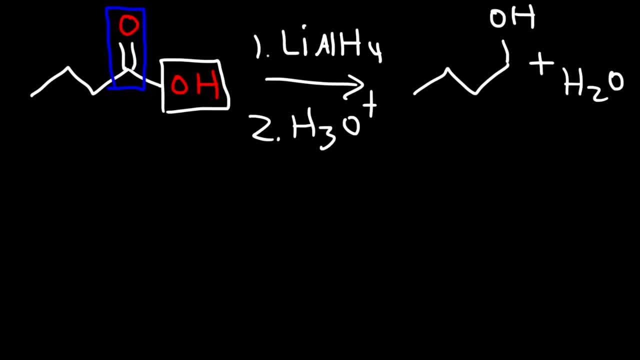 solution, but the end result is that it'll leave is water, which we don't really have to worry about, so the final product will be a primary alcohol. now, what if we have, let's say, an amide functional group? what's going to happen if we reduce it with lithium aluminum hydride? 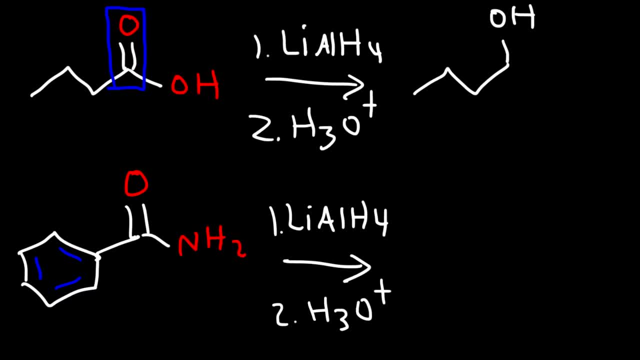 what do you think the major product for this reaction is going to be? in this case, the amide will be reduced to an amine, so the carbonyl group won't be reduced to an alcohol. it's going to be reduced to a CH2 group, and so you're. 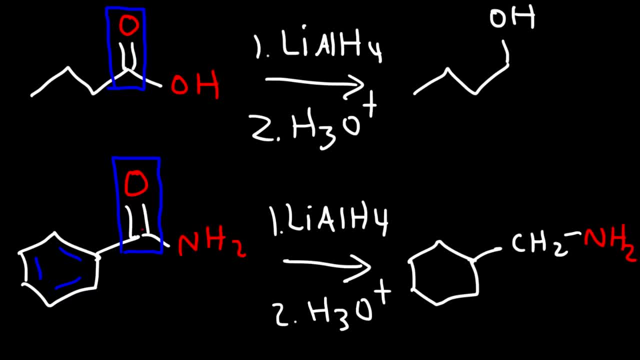 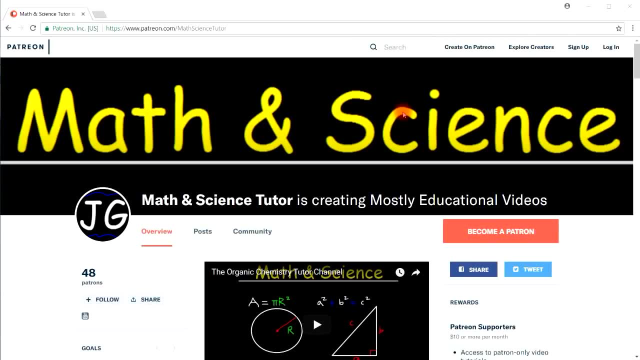 going to get this a primary amine. now, for those of you who might be studying for the organic chemistry finalists final exam, I have a video that can help you and it's on my patreon page. if you go to patreoncom slash math science tutor, you can access that page if you scroll. 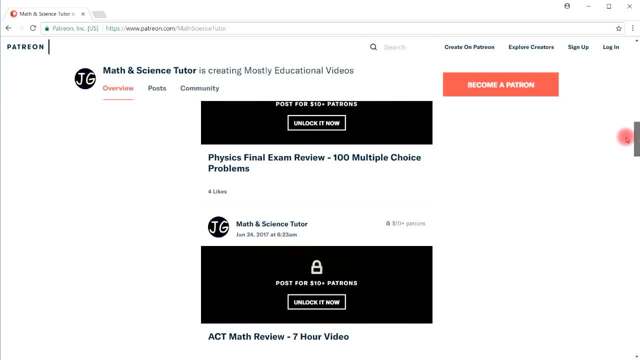 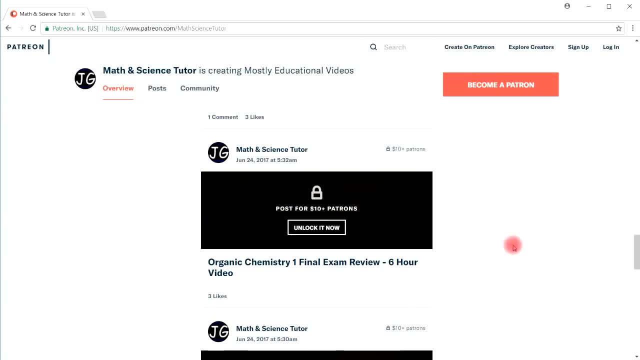 down. there's a lot of other videos I have here too, but let's say, if you're taking the first semester of organic chemistry, I have a six-hour video that can help you with that. if you decide to become a patron now on YouTube, I have a free two-hour trailer version of this video, but if you want the 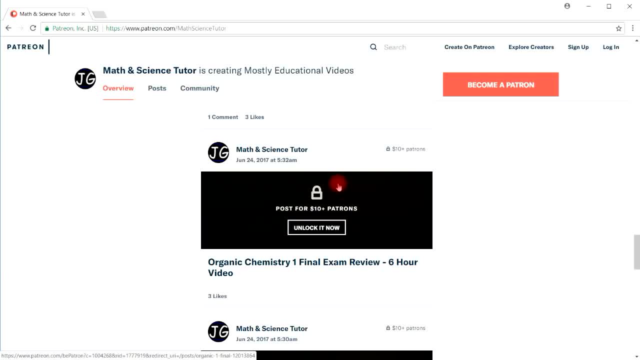 entire six-hour video. you can access it here or on Vimeo as well, and for those of you who are taking the second semester of organic chemistry, I have an eight-hour video that you can access as well, and there's some other stuff here that you could find too. 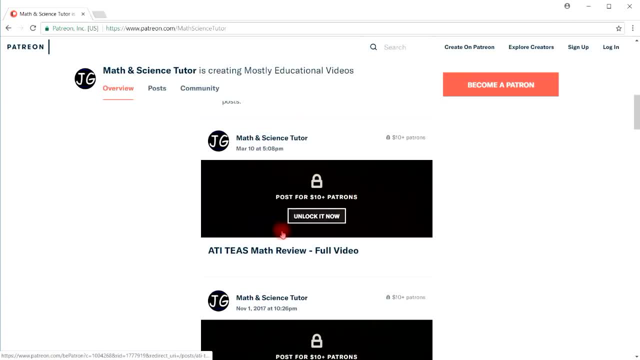 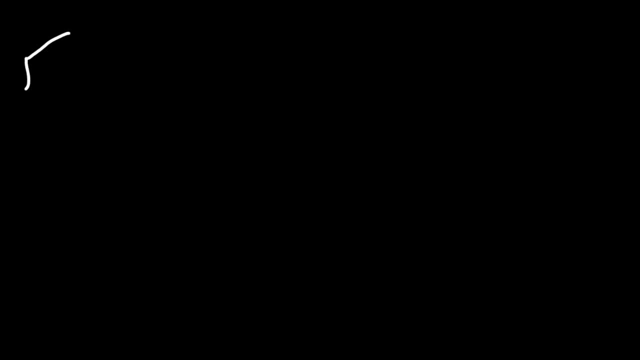 if you're taking gen chem or physics. I have stuff on that as well, so that's it, just in case you're interested. now let's go over some other reactions. what's going to happen if we react cyclohexene with hydrogen gas and palladium over carbon? now you know that. 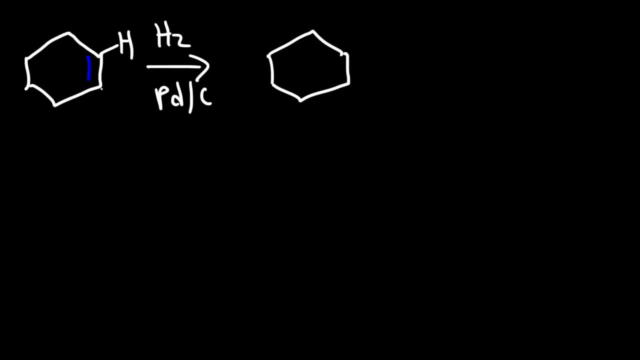 the alkene will be reduced to an alkane by the addition of two hydrogen atoms which are on the same side with respect to each other. now something similar happens if we react, let's say, a ketone, with hydrogen gas, but we're going to use a different catalyst, in this case, the rainy nickel. 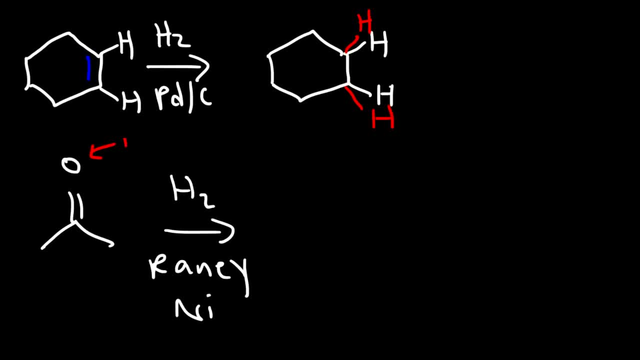 catalyst. so we're going to add a hydrogen on the oxygen and on its carbon. so the end result is that we're going to get an alcohol, which you can represent like this: so here's the hydrogen that was added to the oxygen and here's the hydrogen that was added to the carbon. so we basically add two. 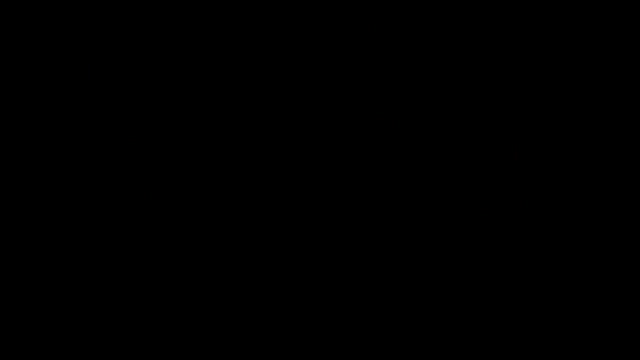 hydrogens across this carbonyl group. now, what about an aldehyde? what if we react it with hydrogen gas using the rainy nickel catalyst? the effect will be the same. we're going to add a hydrogen on the oxygen and on the carbon, so we're going to get a primary alcohol. 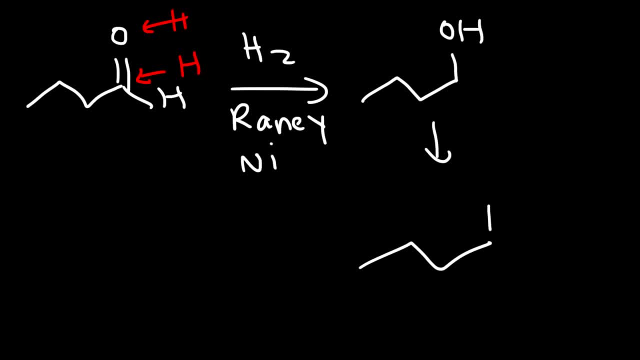 so here's the hydrogen that was added to the oxygen, and here is the hydrogen that was added to the carbon, and here is the other hydrogen that was already present, which you can see here, and so basically, you just add two hydrogen atoms across the double bond, and so you get C with an O, the O has an H and the C 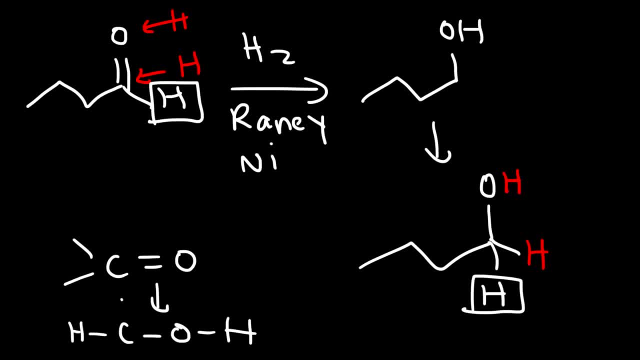 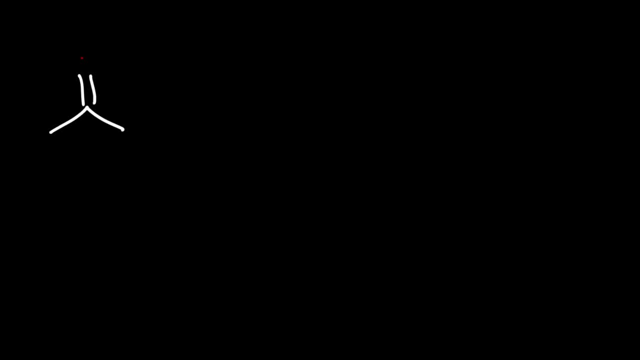 has an H and, of course, the C has two other bonds. so, based on that example, let's say, if we have an imine and we wish to react it with hydrogen gas, with palladium over carbon, what do you think the major product of this will be? so we're going to add a. 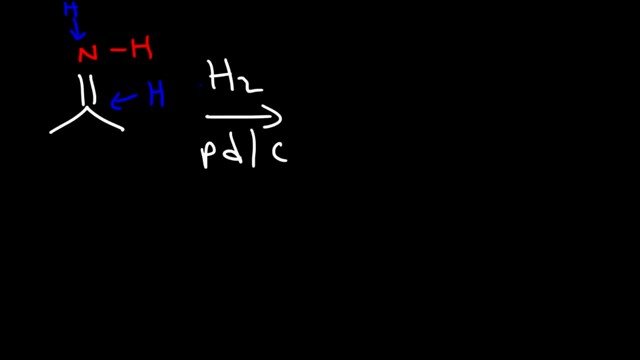 hydrogen across the double bond, so one on the carbon and one on the nitrogen. so now the nitrogen has a total of two hydrogen atoms, and the carbon also has a hydrogen. so the end result is that the imine has been reduced to an amine. now what if we have, let's say, a? 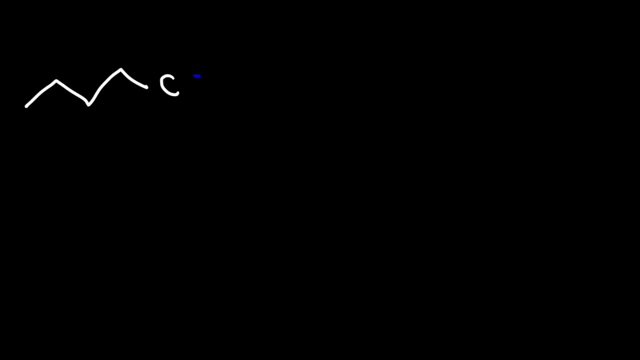 a nitrile. What's going to happen if we react the nitrile with hydrogen gas? Now we need two equivalents of hydrogen gas. Well, once you add the first equivalent of hydrogen gas to a nitrile, the triple bond will go down to the double bond level. 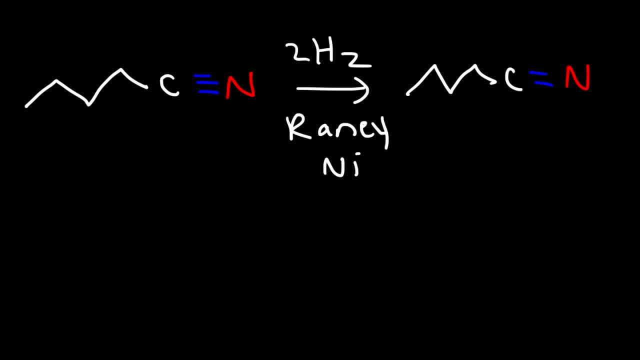 and we're going to add a hydrogen across that triple bond, So one at the carbon and one at the nitrogen. So that's when the first equivalent of H2 reacts with the triple bond. So then once we react it again with another hydrogen gas, 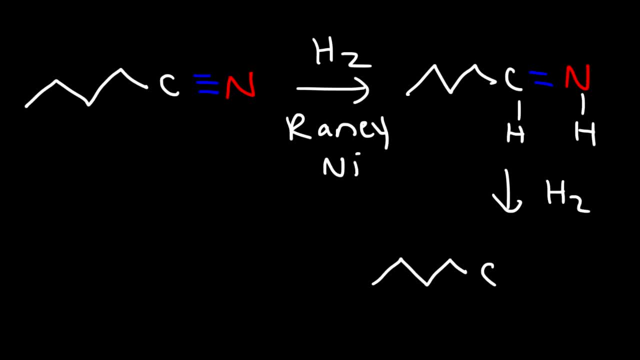 the double bond will go down to a single bond, and so we're going to get an extra pair of hydrogen atoms across that CN bond. And so the net effect of using hydrogen gas with the rhenium nickel catalyst is we convert the nitrile. 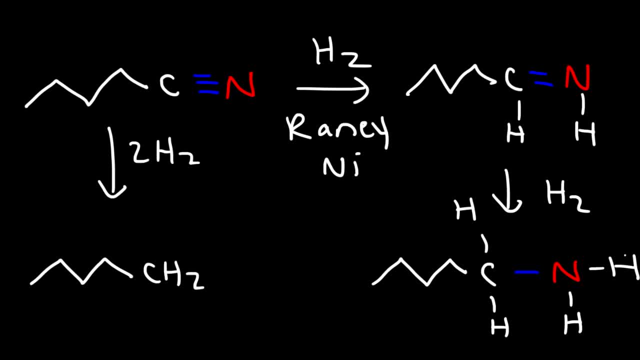 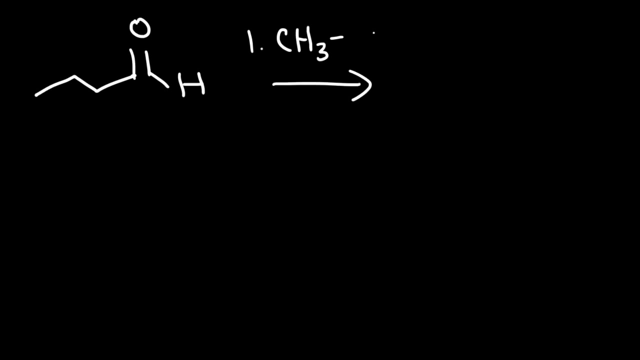 into a primary amine, And so that is the net effect. So that is the reduction of a nitrile into an amine. Now let's talk about the reaction of aldehydes with Grignard reagents. What's going to happen if we react butanol with methyl magnesium bromide? 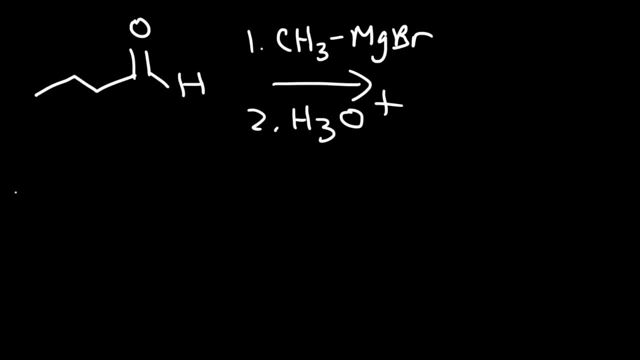 followed by H3O plus. What do you think the major product will be Whenever you have a carbon atom bonded to a metal? that carbon is nucleophilic, And so it will attack the partially positive carbon of a carbonyl group. So right now we're going to get an alkoxide ion with a methyl group added to it, And then, in the next step, we can react it with H3O plus, And so the Grignard reagent can convert an aldehyde or ketone into an alcohol. 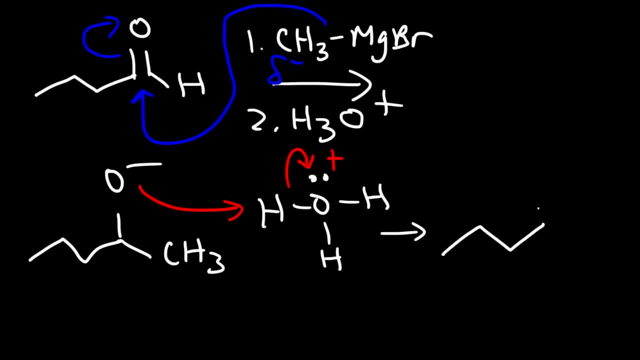 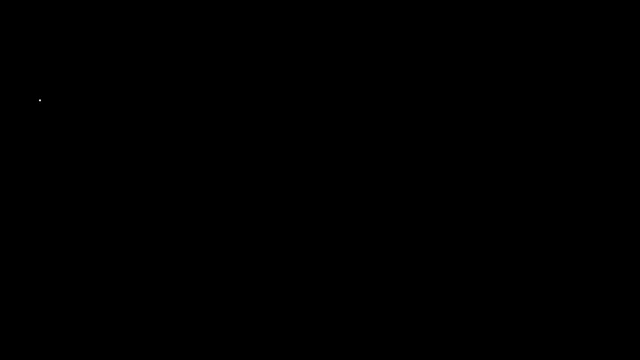 In the case of this aldehyde, we have a secondary alcohol. Now what type of alcohol do you think we'll get if we react the Grignard reagent with a ketone? Well, let's find out. So let's say we have cyclopentanone. 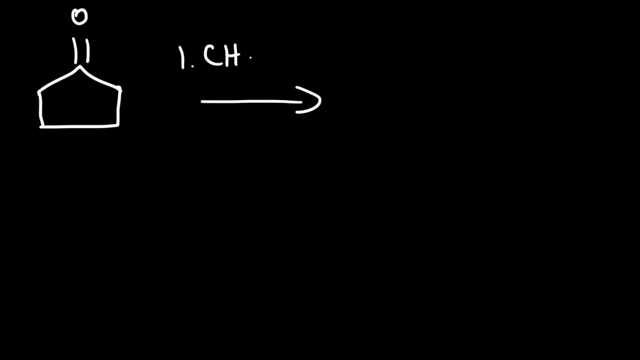 and we're going to react it with ethyl magnesium bromide, followed by H3O plus, So the ethyl group will attack the carbonyl carbon, And so we're going to get an alkoxide ion that looks like this with an ethyl 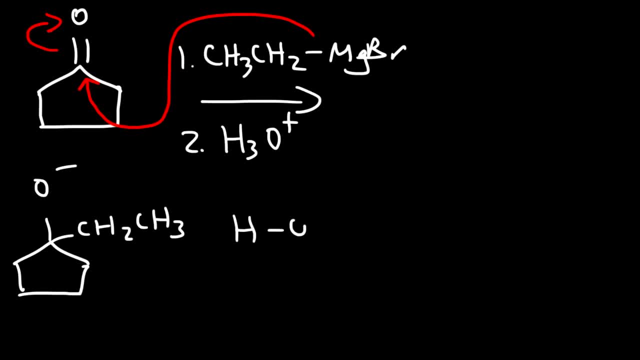 group attached to it. And then, in the last step, we are going to protonate the alkoxide ion, And so, as you can see, the end result is a tertiary alcohol. So the Grignard reagent is useful for converting aldehydes and ketones into 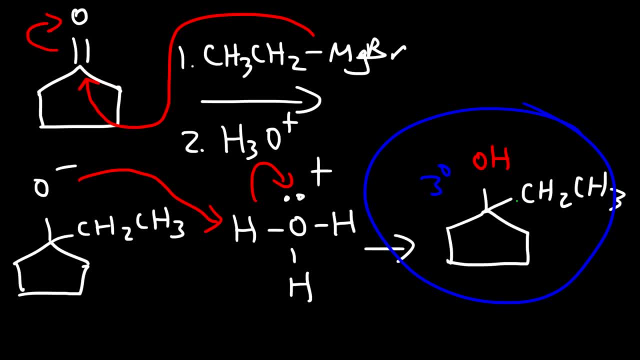 alcohols by the addition of an R group, such as an ethyl group, a methyl group or so forth. Whereas sodium, borohydride, NABH4, and lithium aluminum hydride, they can reduce an aldehyde or ketone into alcohols by the addition of a hydride. 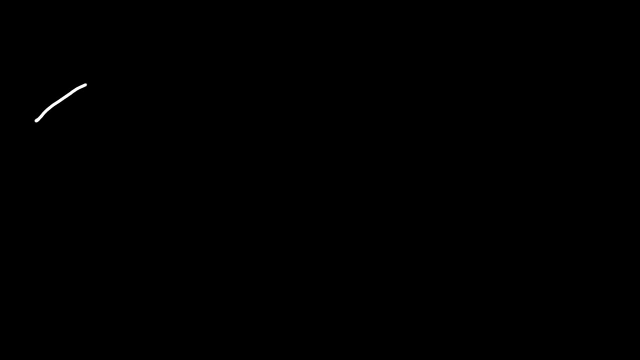 ion. Now let's look at another type of reaction. What's going to happen if we have a ketone and if we react it, let's say, with a primary amine under mild acidic conditions? So to dry your product, what you need to do is remove H2O and then connect the 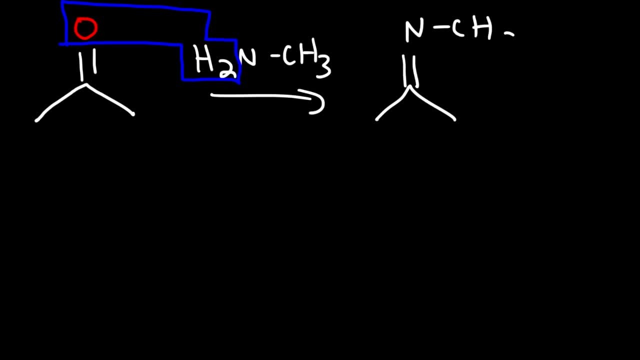 remaining pieces together, So you're gonna get something called an imine. If you react it with ammonia, you'll also get an imine. The key is that there has to be two or more hydrogen atoms on the nitrogen atom to get an imine. If you have one hydrogen on the 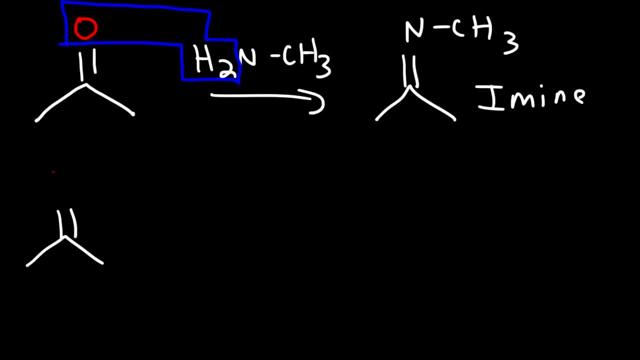 nitrogen. let's say, if you react the ketone with a secondary imine, you're going to get something else. So here is a secondary amine. Let's use a different ketone this time. So instead of getting a double bond between the carbon and the nitrogen, 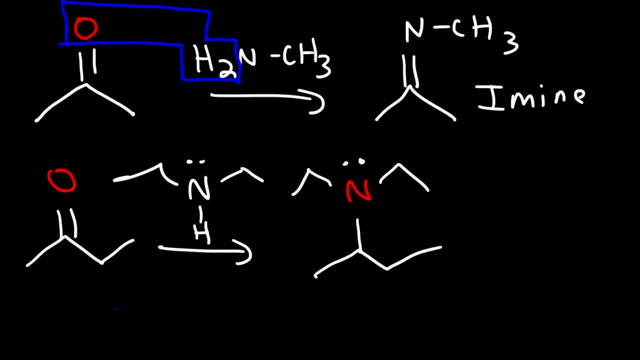 we're going to get a single bond, but we're also going to get a double bond between two carbon atoms. So we have an amine and an alkene. So collectively this is called an anamine or enamine. So that's what you're going to get if you react a secondary amine with a ketone. 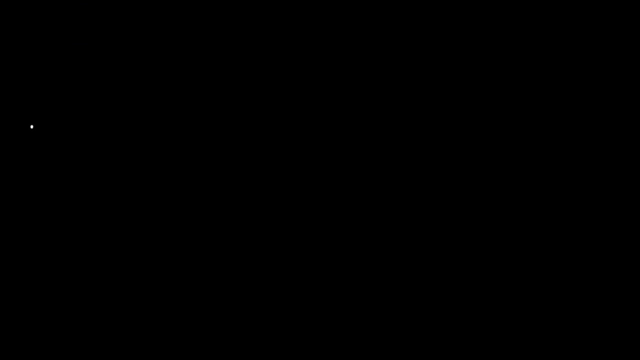 You get an enamine. Now let's go over the mechanism for the formation of an imine. So I'm going to take a ketone and I'm going to react it with NH3.. By the way, all the steps of this reaction. 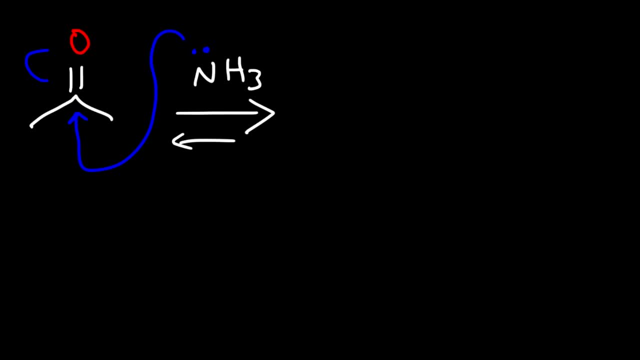 they're reversible. So ammonia is going to attack the carbonyl carbon, giving us an intermediate that looks like this: So right now the nitrogen atom has a positive formal charge And then the oxygen is going to accept a proton from the solution. 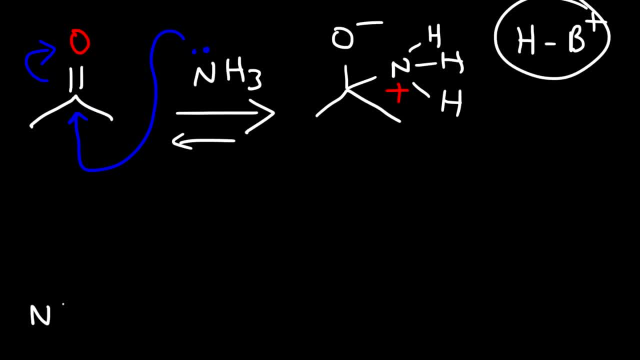 This represents an acid. The acid could be NH4+. It could be H3O+ if we're using water as a solvent. So it's just a generic way of expressing an acid. So the oxygen with a negative charge will take a hydrogen from a weak acid, turning into 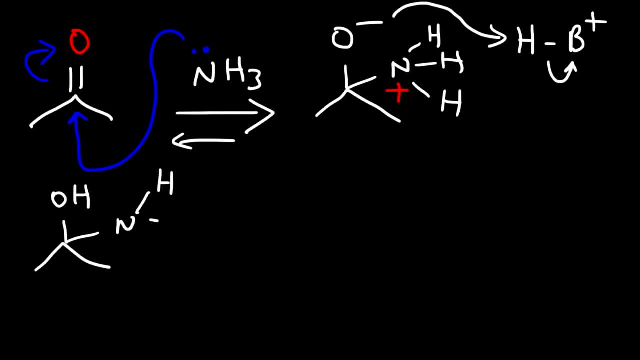 an OH group. Now the weak acid is now a weak base because it lost the hydrogen, and so that base is going to take a hydrogen from nitrogen atom, And so at this point what we have is called a carbonyl amine. In the last step we saw 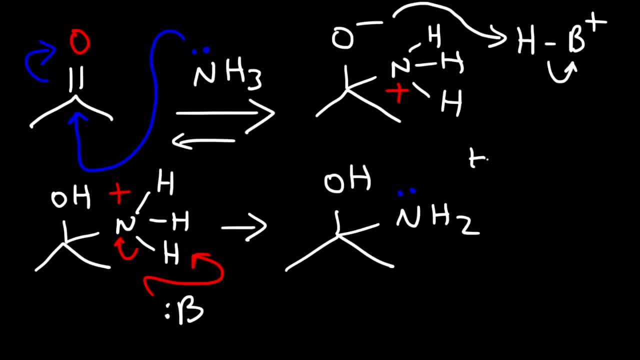 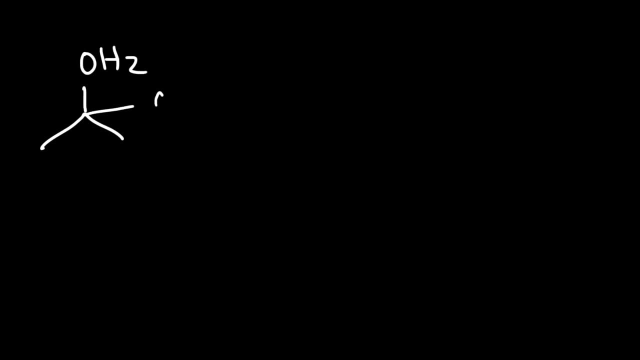 the base took the hydrogen, and so now it's back in its acidic form, and so the OH group is going to accept a proton, turning into a good leaving group, and so this is what we now have. Now the nitrogen atom is going to use its lone period to form a pi bond. 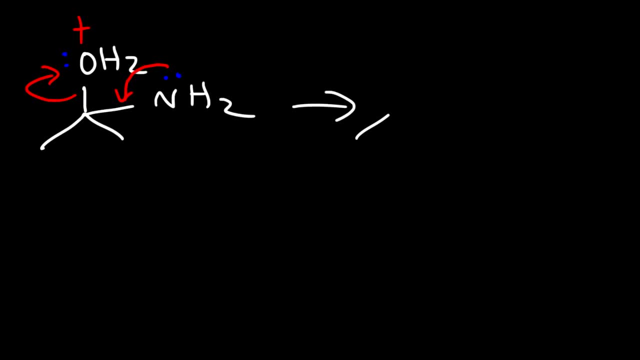 expel in water, since it's now a good leaving group, And so at this point what we have is a protonated amine, So the nitrogen atom has a positive charge, and then we could use the base in a solution to take off a hydrogen atom from the. 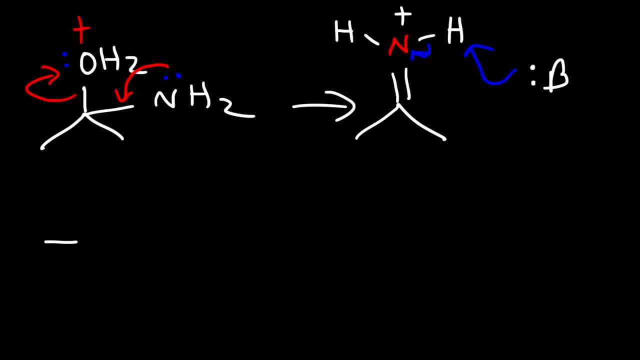 nitrogen atom, And now we have our amine final product, And so that's one way in which you can propose a mechanism for the formation of an amine from a ketone. So now let's go over the formation of the N-amine from a ketone, So we're going to react it with a. 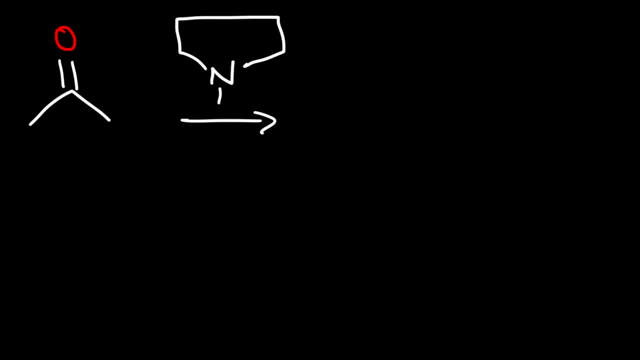 secondary amine which will look like this. So the first thing that's going to happen is that the nitrogen is going to attack the carbonyl carbon just like before, And the conditions is mildly acidic and right now we're going to have a nitrogen atom with 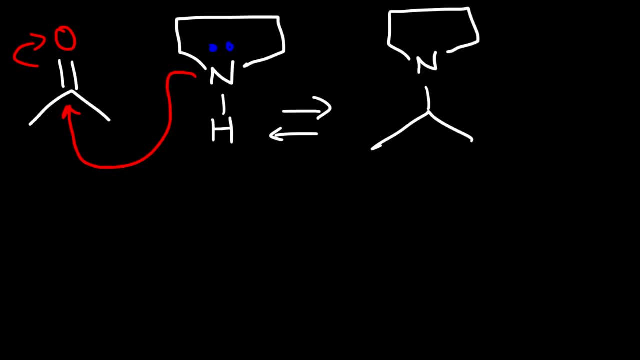 those four carbons. It doesn't have a lone period anymore. It has a hydrogen and we have an oxygen with a negative charge, But the nitrogen now has the positive formal charge, And so in the next step, what we're going to do is react it with a. 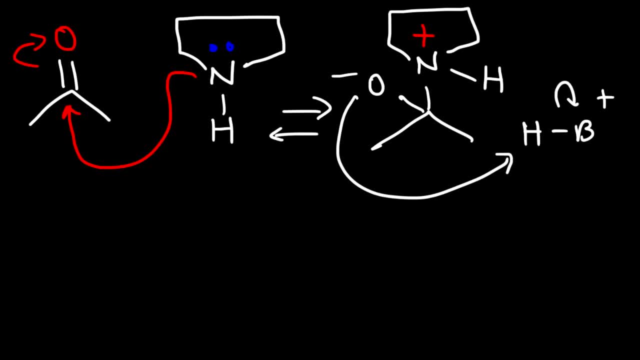 weak acid, We need to add a hydrogen to the oxygen, And so now we have an OH group. We still have the nitrogen with a positive formal charge. The mechanism for the formation of an imine is very similar for the mechanism for the formation of an N-amine, at least in the beginning, But towards the end it's going to. 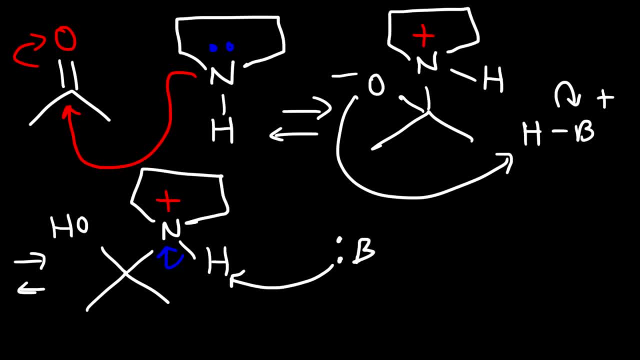 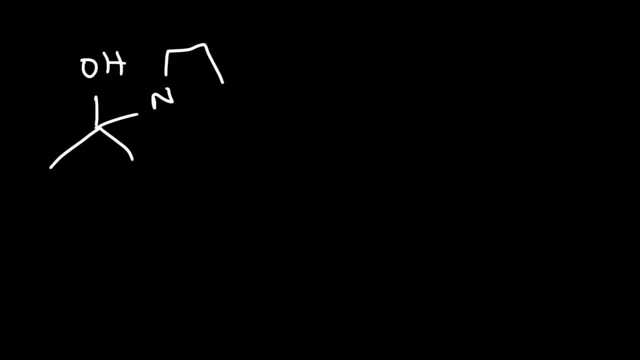 differ. So we need to use a base to take off the hydrogen, And so now we have this, We have our OH group and the nitrogen with a lone period at this time. So now that the base took a hydrogen, it's back in its acidic form And so the oxygen is. 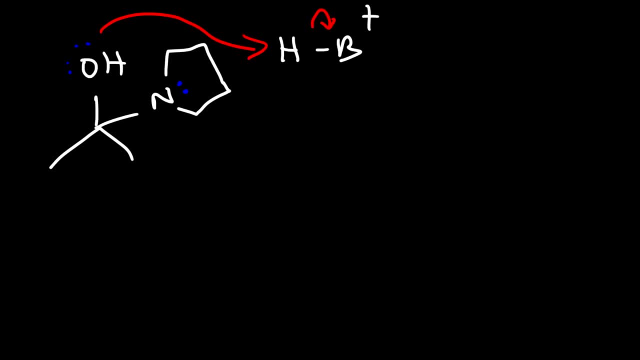 going to grab a hydrogen And every step in this reaction is reversible. so just keep that in mind. And now we have a good leaving group. So once you have the good leaving group- in this case H2O- use the lone period on the nitrogen atom to expel water from this. 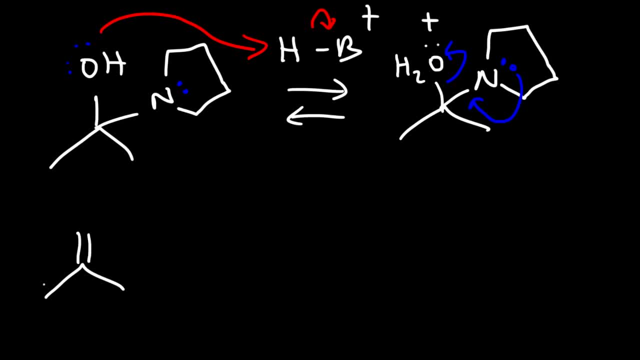 intermediate. So now we have a double bond between a carbon atom and the nitrogen atom, And I'm running out of space here. So now there's a positive formal charge on the nitrogen atom. Now, in the next step, we need to form a carbon-carbon double bond. Now, let's say, we have an extra carbon atom. 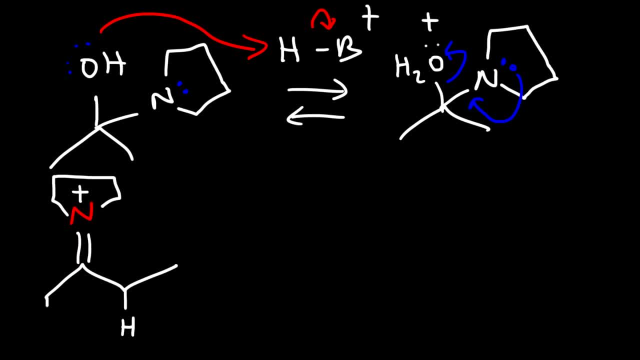 There's two hydrogen atoms that the base can remove. Let me make this a blue hydrogen atom. It can take a blue hydrogen atom or it can take the white hydrogen atom, And so if it takes the blue hydrogen atom, we could form a double bond here, A less stable alkene. Or, if it takes the hydrogen atom, we could form a more stable alkene, And so the base is going to go to the double bond. or we can take the blue hydrogen atom and we can form a even boosted hydrogen atom. So we don't get any carbon-carbon double bond on that part of thisends here. 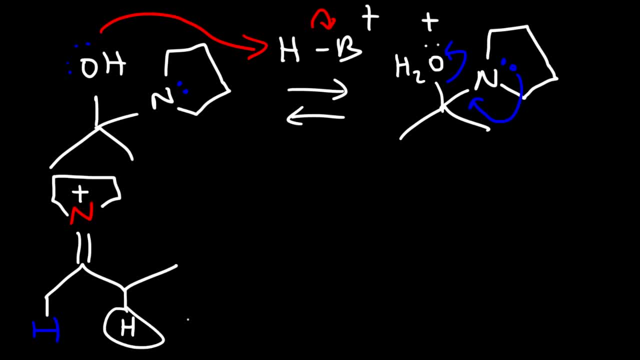 We can't get it from one side to the other end When we leave the flavor And again what we have here is we're gonna pour liquid at the bottom. Let's that double bond to go for the white hydrogen atom, because it leads to the more stable 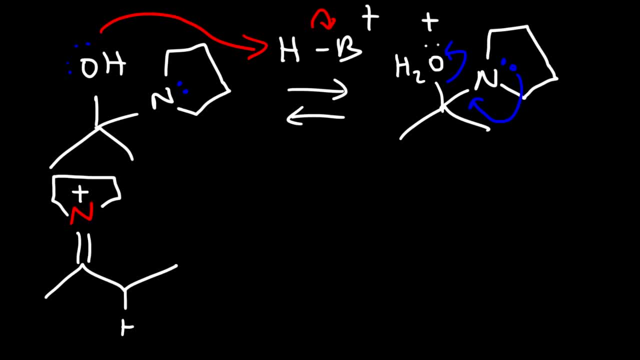 product. So keep that in mind. if you have an unsymmetrical ketone, The more stable enamine will be formed. So we're just going to take off this hydrogen and we could use this base that was just formed in the last step. So it's going to grab. 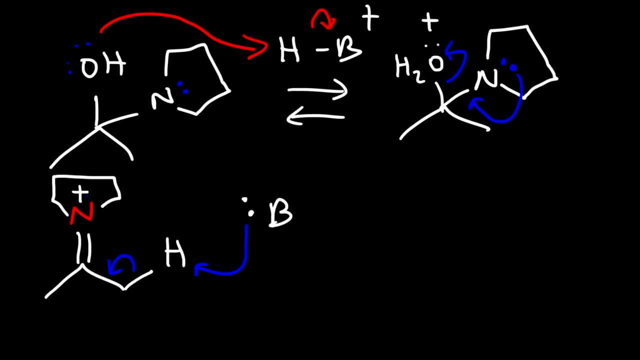 the hydrogen, The carbon-hydrogen bond, will break, forming a pi bond, breaking this pi bond in the process, And so now we have the enamine, which looks like this: And so that is the mechanism for the formation of an enamine from a. 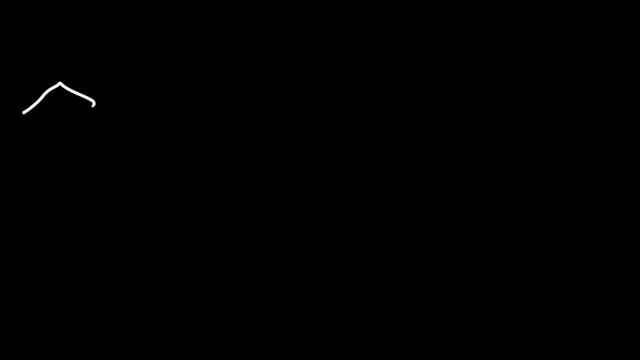 ketone. Next we're going to discuss a reaction called reductive amination and basically it converts ketones into amines. So first we're going to react with ammonia and this is going to give us an imine. So water is a side product. You need to take away the oxygen. 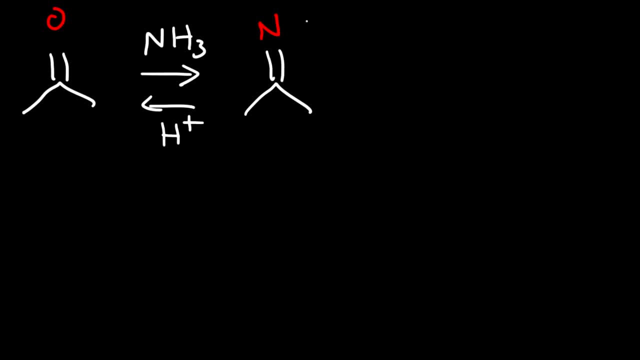 and two hydrogen atoms from the nitrogen atom, which leaves behind one hydrogen atom, And so now we have the imine product, And then we could reduce the imine using hydrogen and palladium over carbon into an amine, And so that process, the conversion of a ketone into an amine, is reductive amination. So here's. 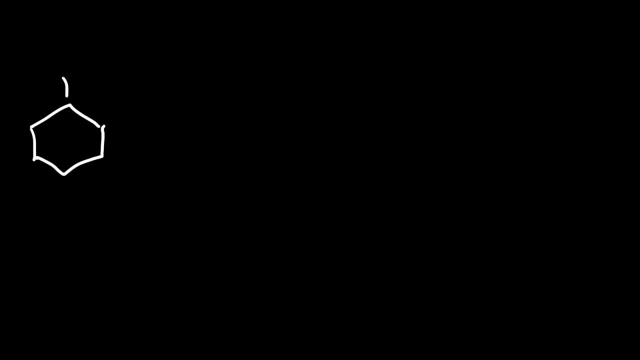 another example. Let's say, if we have cyclohexanone and let's react it with a primary amine under mild acidic conditions, And so let's use methoamine, And so this is going to give us an imine. Now, if you take away water, the two hydrogens and the oxygen, you'll be left. 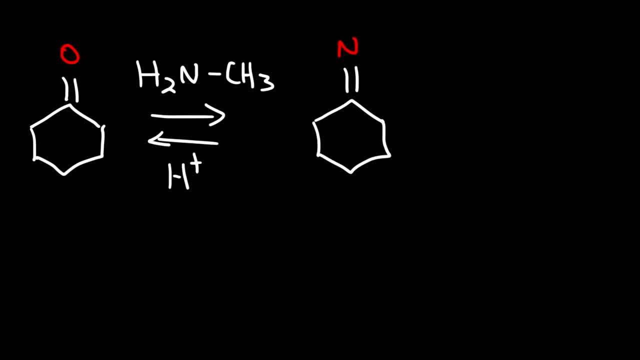 with the R group attached to the nitrogen atom, And then we could reduce it with sodium cyanoborohydride, and a double bond will be reduced to a single bond, giving us a secondary amine. So next up, we're going to have two methyl cyclohexanone, and let's react it. 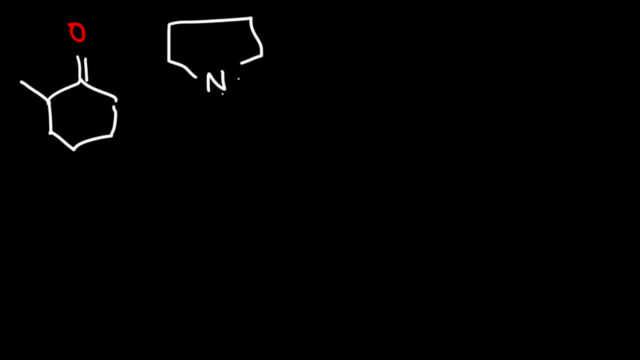 with a secondary amine under mildly acidic conditions. So we know this is going to give us an N-amine. So we're going to have a carbon-nitrogen single bond and a carbon-carbon double bond. So should we put the double bond on the left side or on the right side? The 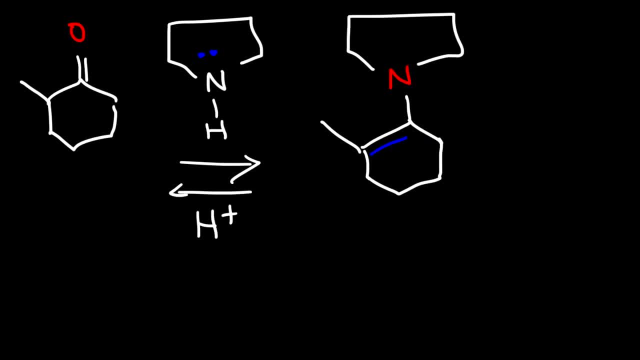 double bond is going to go on the side that makes it more stable, that is, with the R group on the left. So now we have the N-amine and then we're going to reduce it with sodium cyanoborohydride, And so the double bond will be reduced into a single bond. 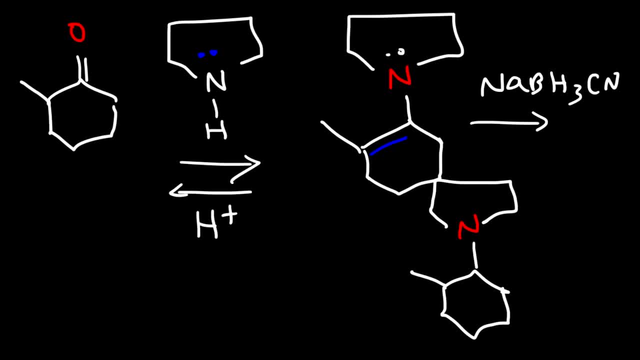 So the final product for this reaction looks like this. So this time we have a tertiary amine as opposed to a secondary or primary amine. Now let's talk about the second product. Let's talk about the reactivity of aldehydes and ketones. 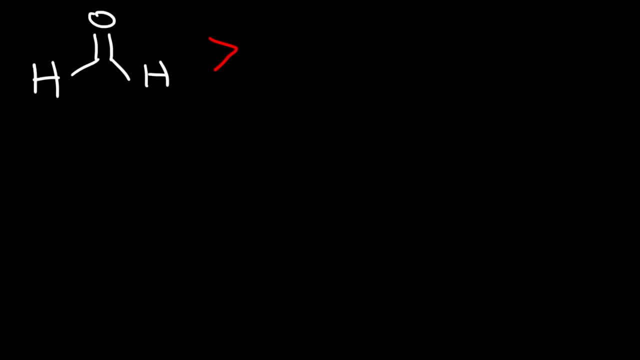 Formaldehyde is more reactive than acetaldehyde And acetaldehyde is more reactive than propanone, So aldehydes are more reactive than ketones. The reason why ketones are less reactive is for one: you have these bulky CH3 groups, which 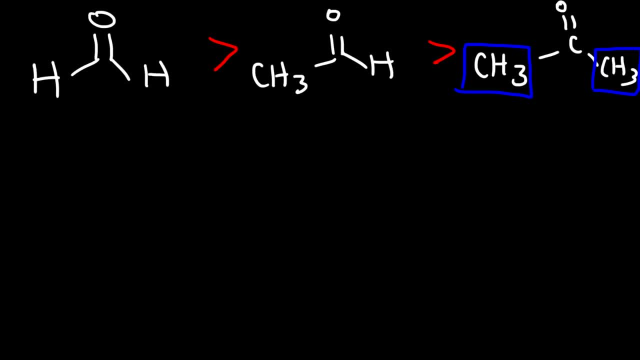 hinders the reaction of acetaldehyde. And also those CH3 groups are electron donating groups, and so they donate electron density to the electrophilic carbonyl group, making it less electrophilic, And so that's why ketones are less reactive than aldehydes. 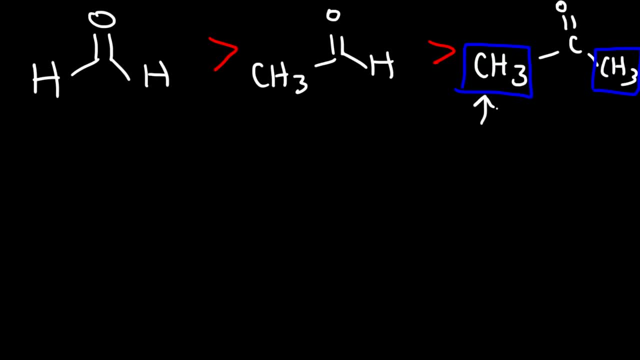 It's due to the steric effects of the methyl groups and also the fact that they donate electron density to the carbonyl group. Let's say, if you were to react formaldehyde with water, Formaldehyde is highly reactive towards water and so it's going to form a hydrate which 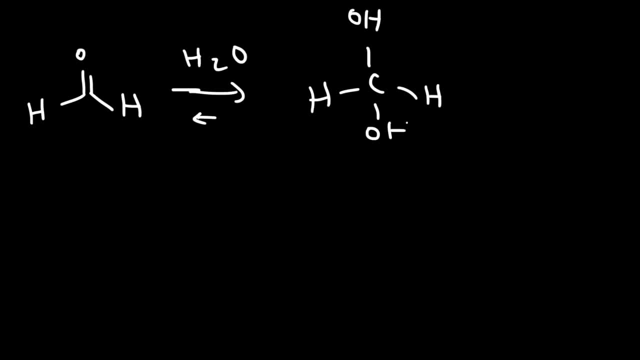 looks like this And notice that we have a bigger arrow towards the right. Now, if we take acetaldehyde And react it with water, And if we take acetaldehyde And react it with water, This reaction is fairly reversible, but we can get the hydrate and aldehyde. 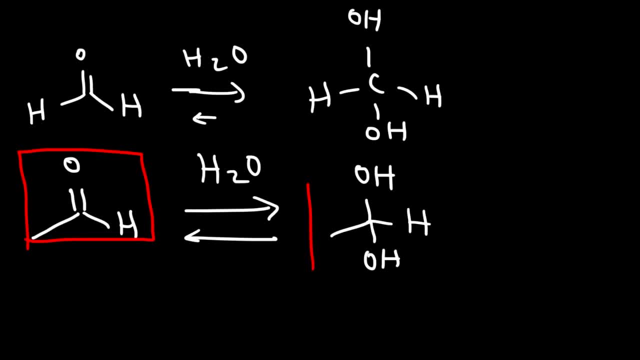 Both of them will exist in a solution in relatively equal amounts. Now the ketone is not really reactive of water. A small amount will convert into the hydrate form, but the majority of it will stay in a ketone form. So ketones are less reactive to water and other nucleophiles than aldehydes. 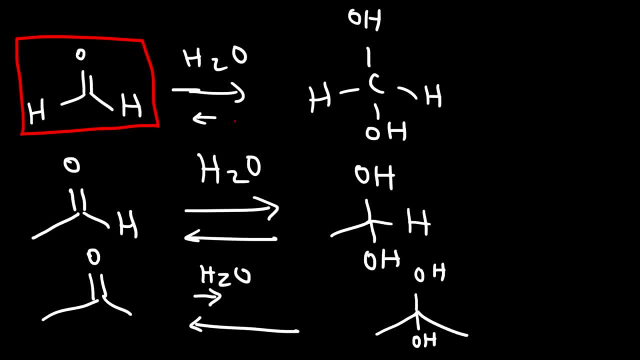 So, as you can see, formaldehyde will virtually completely be converted into the hydrate form. Only a very, very small amount will stay in the formaldehyde form, Whereas acetaldehyde- both of these will exist in a significant amount in equilibrium when water is present. 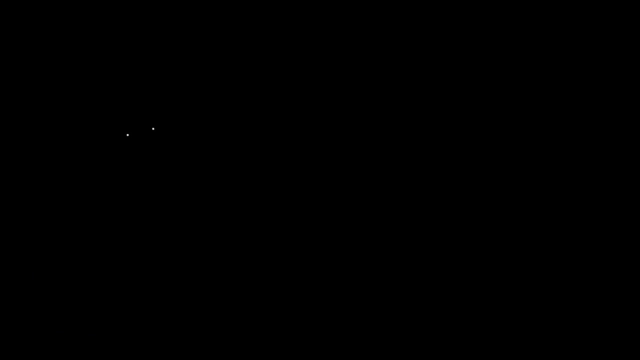 And the ketone. It really doesn't want to react with water. Now consider this reaction between an aldehyde and an alcohol. instead of water, So let's use methanol And we'll need an acid catalyst. So in the first step, we're going to get a hemiacetal. 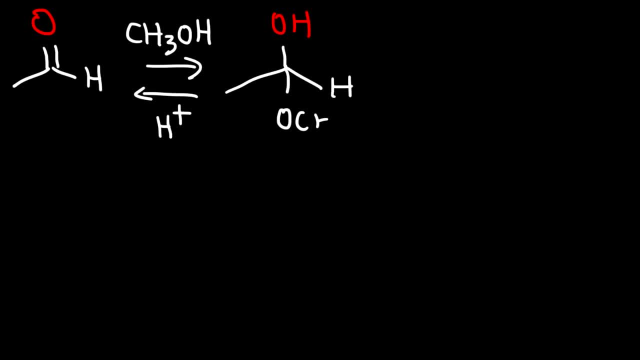 Which is basically a carbon with an OH group and an OR group, So that's a hemi. And then, if we react it with another methanol molecule, we can get an acetal where we have two OR groups instead of one. Now, let's say, if we have an acetal, 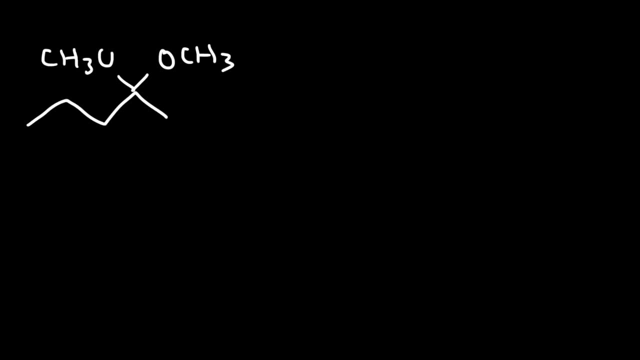 Okay, What's going to happen if we react it with H3O plus With excess water? under acidic conditions you can go back from the acetal group into a ketone. So this reaction is controlled by equilibrium. So if you add water, you're going to go in this direction. 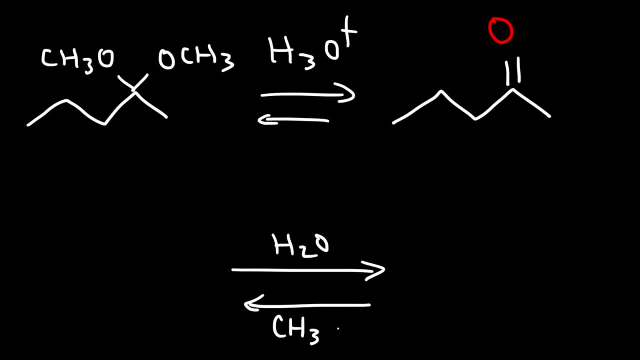 But if you add excess alcohol, you're going to go in this direction. So if you add water, you're going to go in this direction, But if you add excess alcohol, you're going to go in this direction. Under acidic conditions, you're going to go back to the acetal form. 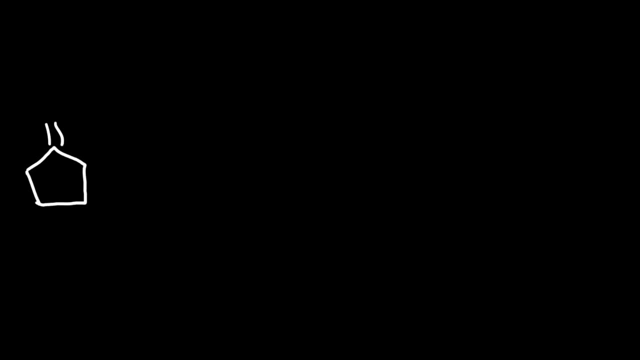 Now let's say we have cyclopentanone and we wish to react it with ethylene glycol. What is the major product of this reaction? So what we're going to get is a protecting group. So we have two alcohol functional groups, but in the same molecule. 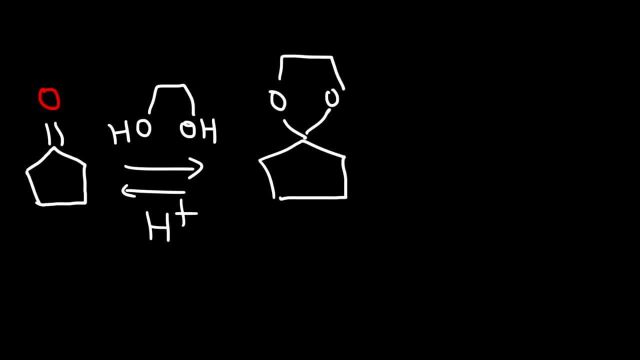 So we're going to get an acetal that looks like this, And it serves to protect the ketone from nucleophiles. Now, to get rid of the acetal protecting group, we just need to add H3O plus, And this will convert it back into the ketone form. 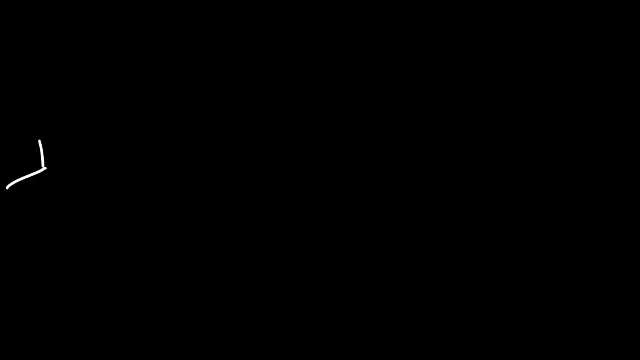 So let's say if Okay, Okay, Okay, We have a molecule that looks like this, So this molecule has a ketone functional group and an ester functional group, What reagents do we need in order to synthesize these three products? 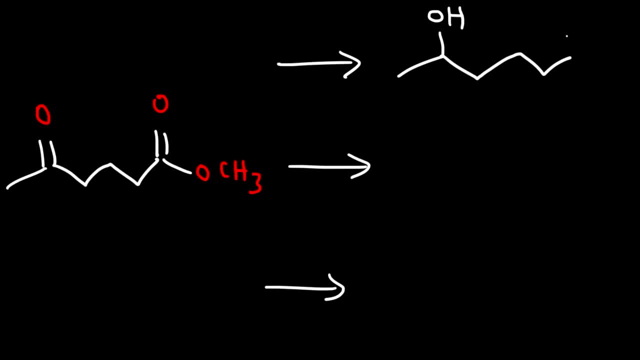 Let's say, if we want to reduce the ketone but not the ester, how can we do so? What reagent do we need to do that? Or let's say, if we want to reduce everything- The ketone and the ester- 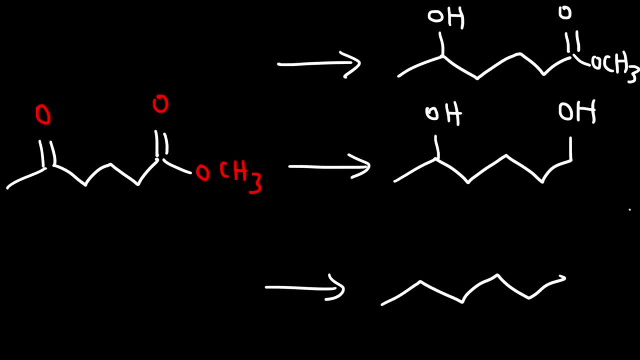 How can we do that? Or what if we want to reduce the ester but not the ketone? What reagents do we need to make these three products? So go ahead and feel free to pause the video. Try these examples. So for the first one, we need to use sodium borohydride. 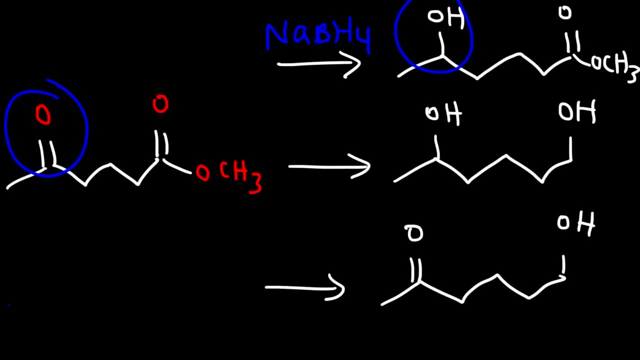 Because this will reduce the ketone and the ester. It will reduce the ketone into an alcohol, but it's not strong enough to reduce the ester, So the ester will be unaffected. Now for the second example. we need to use lithium aluminum hydride because it's a strong 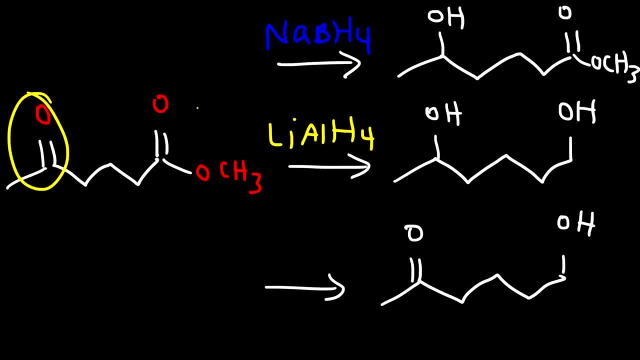 reducing agent. It will reduce the ketone into an alcohol and it will reduce the ester into an alcohol. Now for the last example. we want to reduce the ester but not the ketone, And so in this case, we need to use a protecting group. 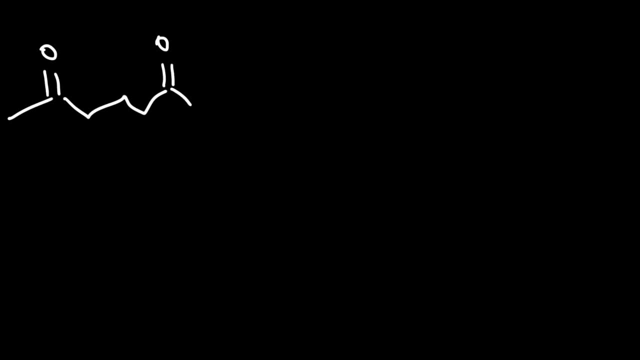 So let's go over this reaction. The ketone is more reactive to nucleophiles than the ester. The ester has an electron donating group, And so the lone pairs on the oxygen can form a resonance structure that makes the carbonyl. 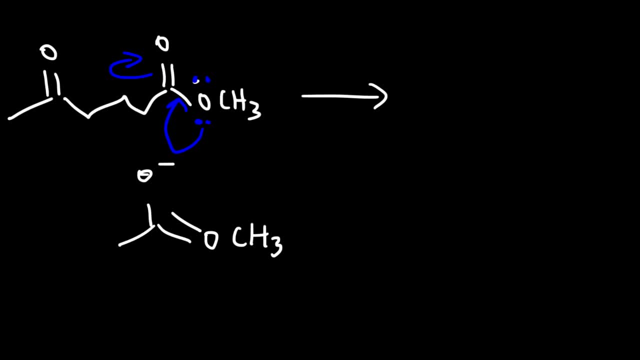 carbon less nucleophilic, You can see, in this form, So it can donate electron density into the carbonyl carbon. So the first thing we need to do is react the ketone with ethylene glycol, And so this will protect the ketone from nucleophilic addition reactions. 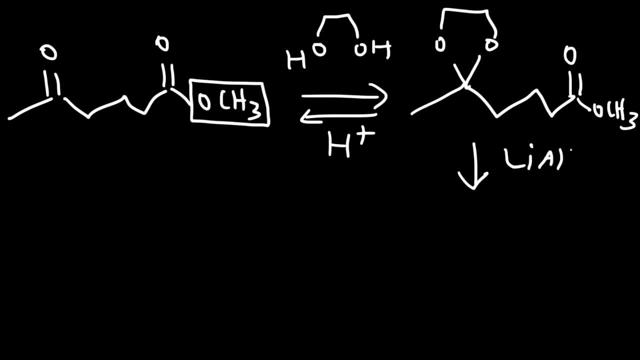 So now we can reduce the ester with lithium aluminum hydride. Okay, Turn it into an alcohol While the acetyl group remains unaffected by lithium aluminum hydride. And then we can remove the protecting group with H3O plus converting it back into a ketone. 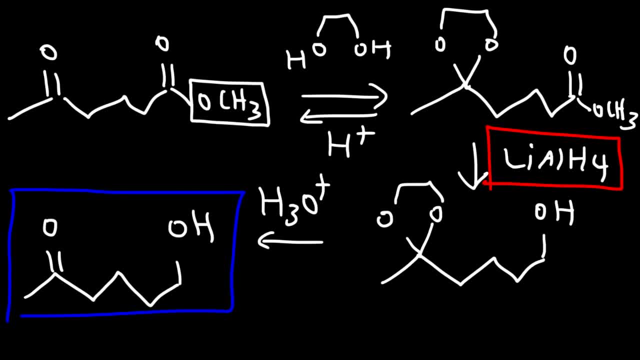 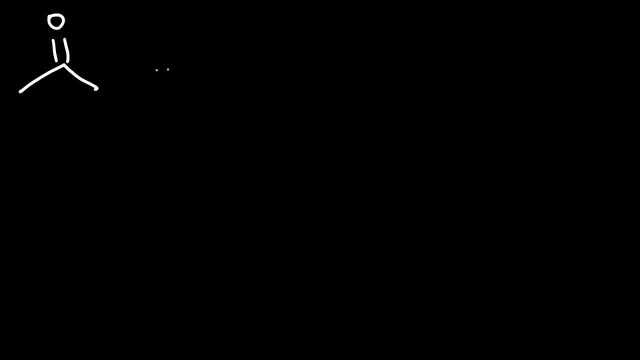 And so that's how we can reduce the ester, but not the ketone, by the use of a protecting group. Now, Earlier in this video, we mentioned a reaction between a ketone and methanol, And this can give us an acetyl which looks like this: 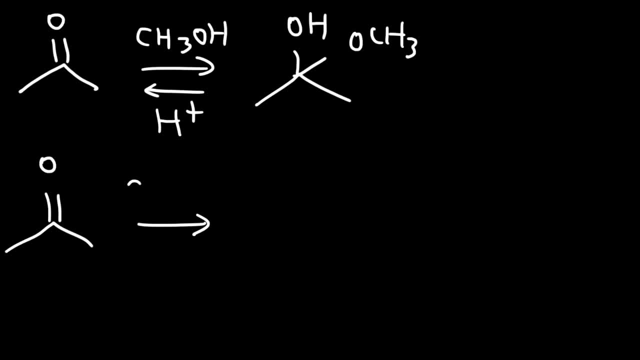 So what if we have a ketone and let's say, we react it with, instead of an alcohol, a thiol, under acidic conditions? Well, we're still going to get the OH group, Okay, So Okay, But instead of an OCH3 group, we're going to get an SCH3 group. 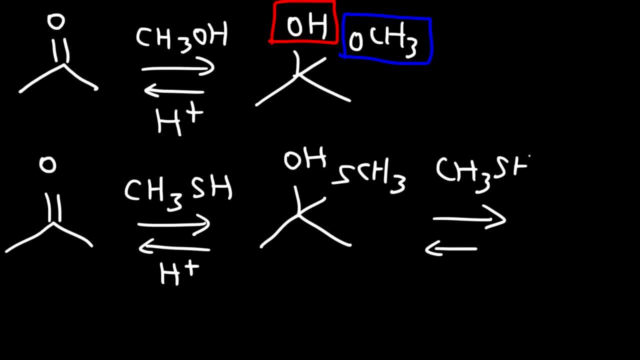 And then if we add another thiol molecule to this, we can remove the OH group and replace it with another SCH3 group. So adding the thiol will drive the reaction to the right, But if we add an H3O plus or water with H plus it's going to cause the reaction to. 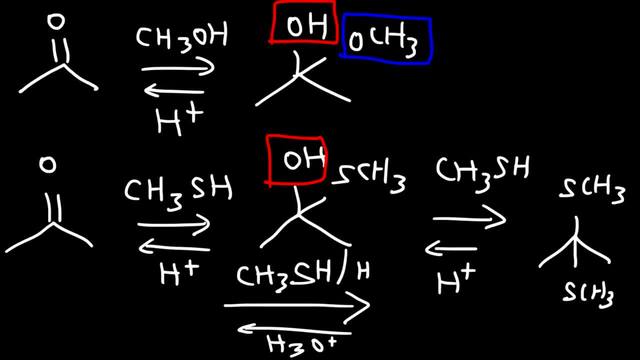 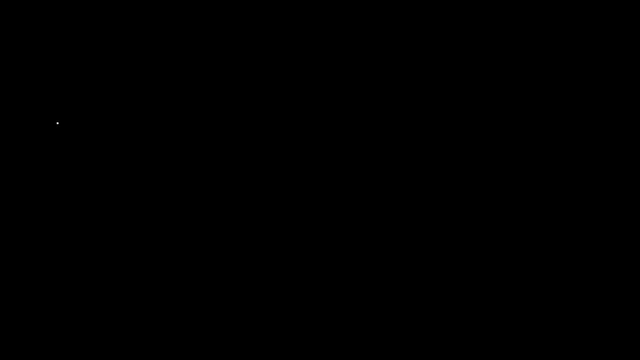 go to the left, So we need to add an acid catalyst to go in either direction. Now, let's say, if we have cyclopentanone, but we wish to add a thiol that looks like this: Okay, So. So we have a molecule that contains two thiol functional groups. 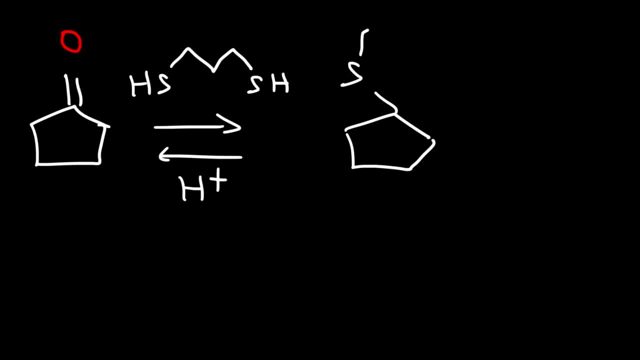 So we're going to get another type of protecting group that looks like this. But we can do some different stuff with this type of protecting group. For instance, if we react it with hydrogen gas using the rainy nickel catalyst, we can completely get rid of all of the sulfur atoms and replace it with hydrogen atoms. 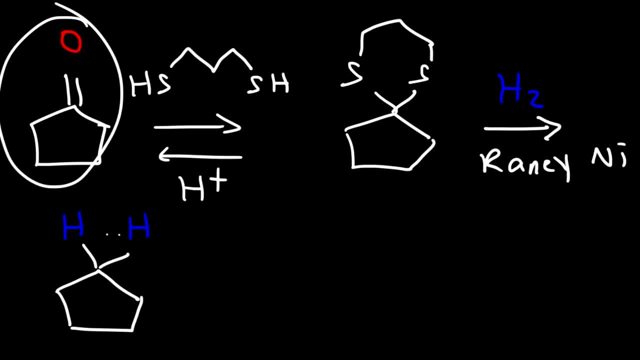 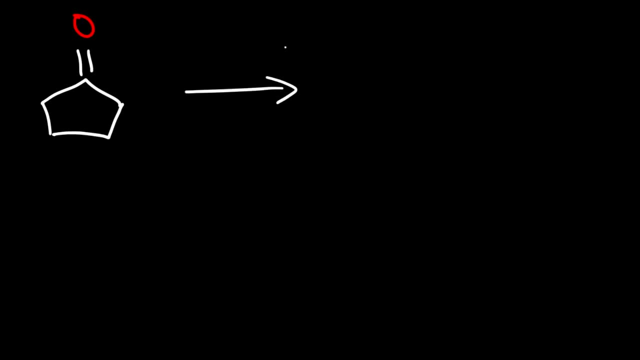 So the net effect is that we converted a ketone into an alkane under mild acidic conditions. Now there are some other ways in which we can reduce a ketone into an alkane. Another reaction is the Clemson reduction reaction, which involves the use of zinc with 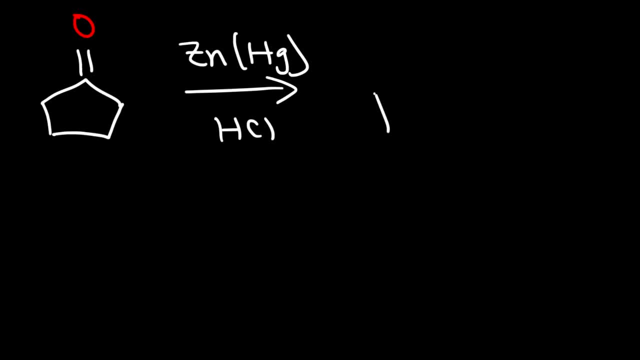 mercury under acidic conditions. Okay, But these conditions are strongly acidic. So the end result is the conversion of a ketone into an alkane by the addition of two hydrogen atoms. Another similar reaction is the Wolff-Kishner reaction, which occurs under strongly basic 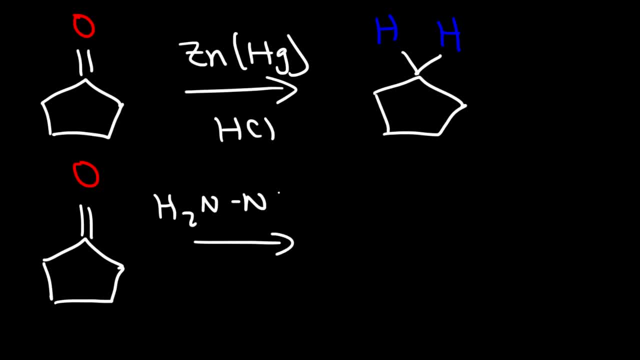 conditions. The reagent is hydrazine, H2N and H2., Which can be written as N2H4. So you might see it like that, And you need a strong base with heat to make this work, And so the end result is the same. 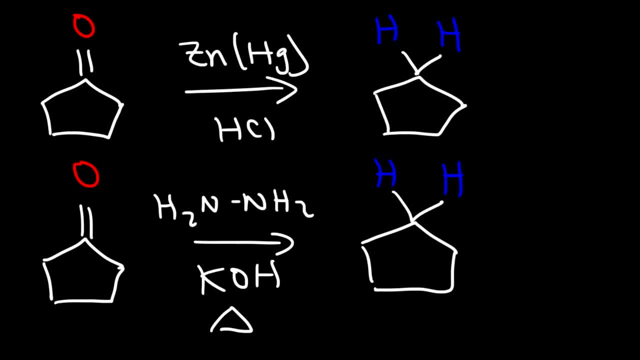 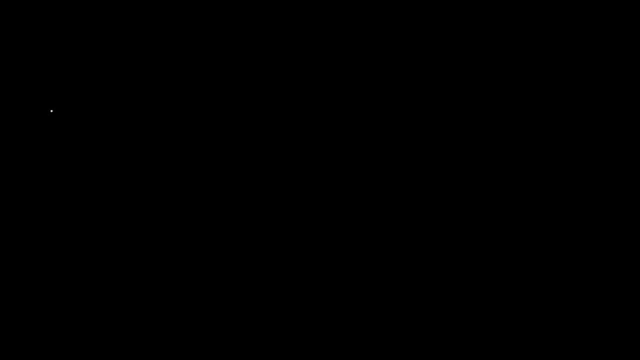 It converts the ketone into an alkane. It completely reduces it into cyclopentane. Another reaction that you need to be familiar with is the reaction of aldehydes with the silver cation. So let's say we react this particular aldehyde with Ag complex with ammonia in a basic solution. 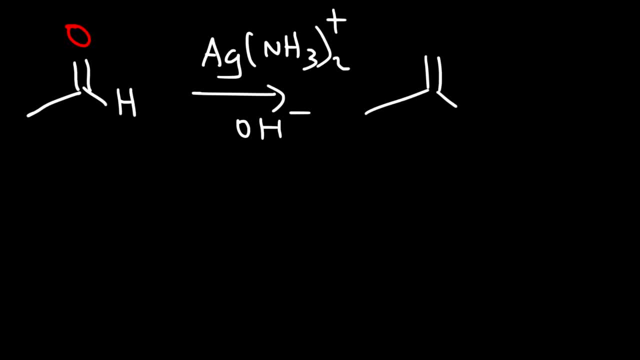 Aldehydes are very sensitive to the silver cation, and so it's going to be oxidized into a carboxylate ion. Under basic conditions, this will be deprotonated, but if, in the second step, you decide to acidify the solution, 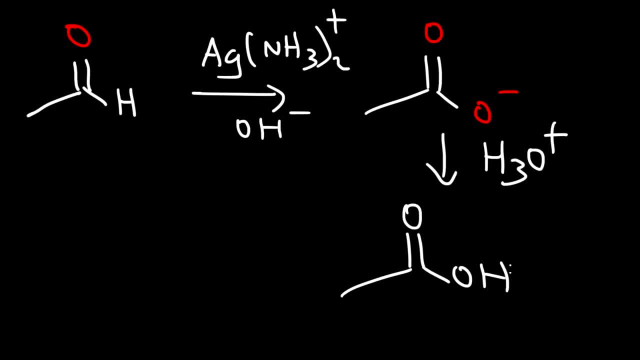 You can convert it into a carboxylic acid. So here's another example. Let's say, if we have cyclopentane carbide and let's react it with silver oxide and water, So in this case the silver is in a plus one oxidation state, and so the aldehyde will be. 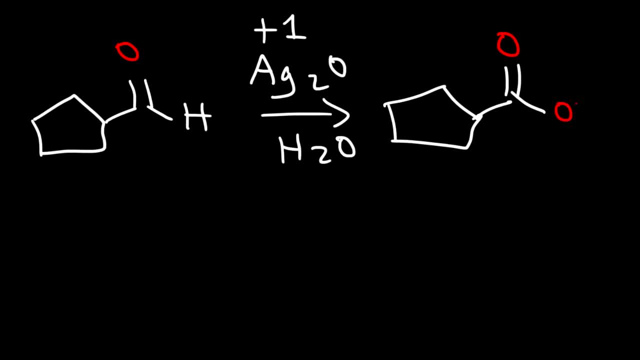 converted into a carbide. So in this case, the silver is in a plus one oxidation state, and so the aldehyde will be converted into a carbide. So in this case, the silver is in a plus one oxidation state, and so the aldehyde will be. 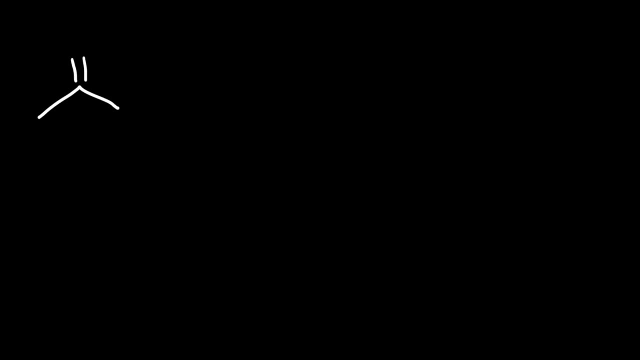 converted into a carboxylate ion. In the next reaction we're going to talk about the formation of a cyanohydrin from the reaction of hydrocyanic acid with a ketone. So the carbonyl group will be reduced to an OH group by the addition of a cyanide ion. 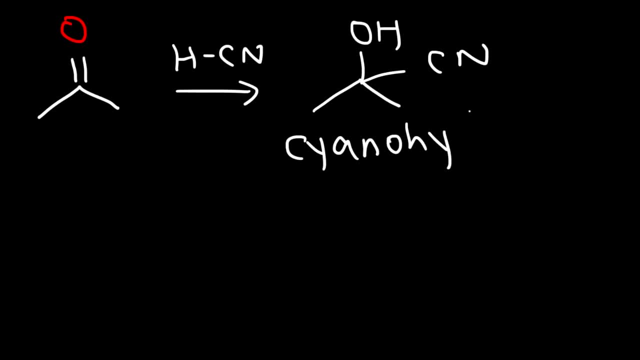 And so this is a cyanohydrin. Now let's go over the mechanism for that reaction. So in the first step, the ketone reacts with the cyanide ion, and so this is a very strong nucleophile, and it attacks the carbonyl carbon, giving us this intermediate. 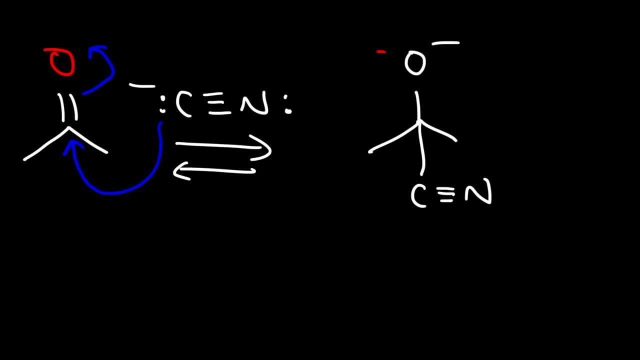 Now, this first step is reversible, because this oxygen can reform the ketone, expelling the cyanide group. Now, in the next step, the oxygen with negative charge is going to take a hydrogen from HCN, regenerating the cyanide ion, And so this is our final product. 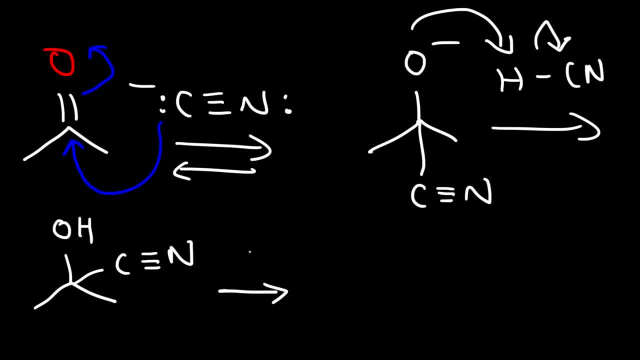 So we get a cyanohydrin. Now, if we react the cyanohydrin with H3O plus, The nitrile will react with H3O plus, And so this is our final product. So we get a cyanohydrin. Now, if we react the cyanohydrin with H3O plus, The nitrile will react with H3O plus, The nitrile will react with H3O plus, And so this is our final product. So we get a cyanohydrin. 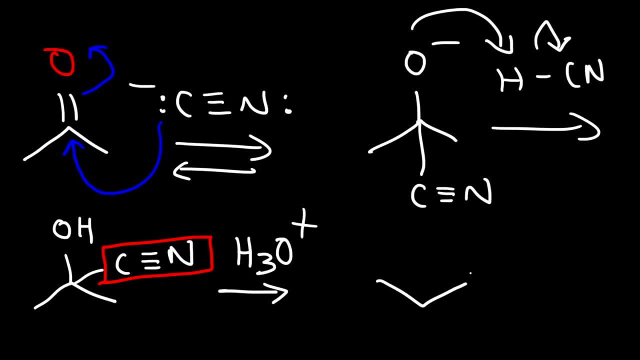 We are going to react with H3O plus. So this is our final product. We will be converted into a carboxylic acid, And so we are going to get a carboxylic acid. We have an OH group on this carbon and we have a methyl group as well. 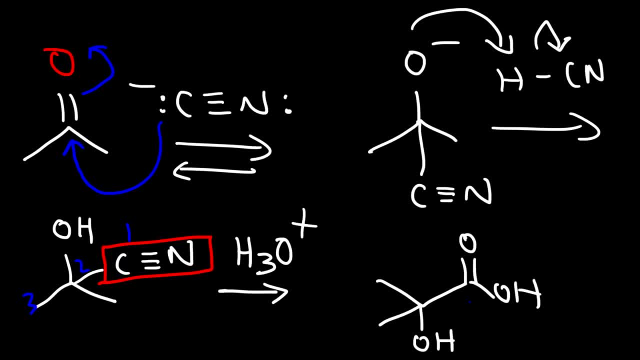 So let's call this carbon 1,, 2 and 3.. So the carboxylic acid group is on carbon 1 where the nitrile was On carbon 2. we have an OH group And we have a methyl group. 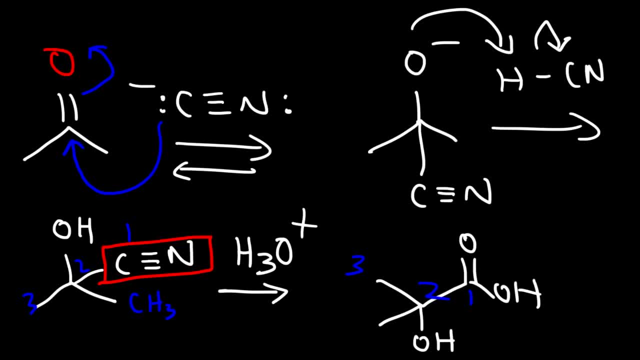 We are going to be converting this into a carbosilic acid And then this is going to be carbon-3.. So that is an alpha-hydroxycarbosilic acid. The hydroxy group is on the alpha carbon. 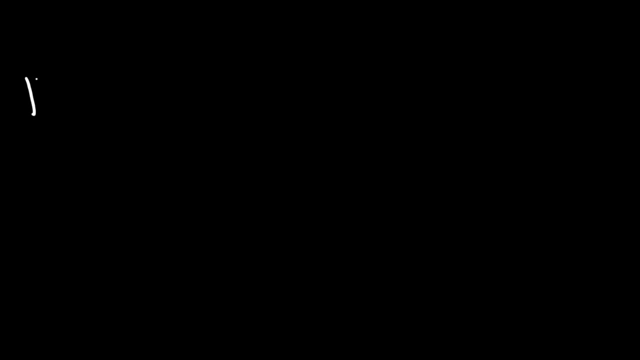 This is the beta carbon. So next up in our list of stuff to talk about is the Wittig, or rather the Wittig reaction. So here we have cyclopentanone And we're going to react this stuff with something called an illid. 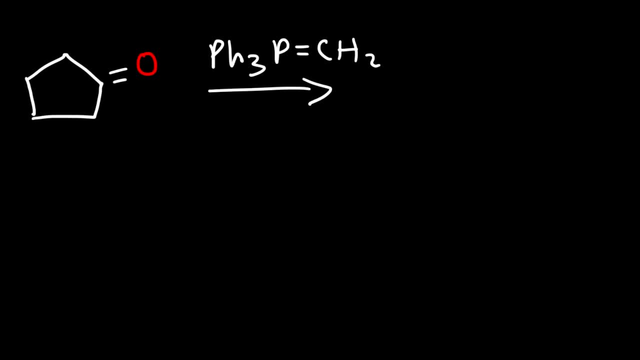 Who came up with these names? What's going to happen here? What is going to be the major product? in this example, All we need to do is basically replace the oxygen with the CH2 group, And so the Wittig reaction is very useful for converting ketones into alkenes. 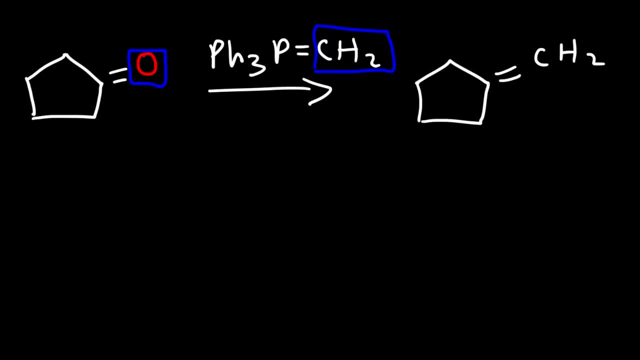 And so this is going to be the major product. Now let's look at another example. So let's say we have another ketone, a very simple ketone, And we're going to react it with an illid, But this illid is going to look a little different than the other one. 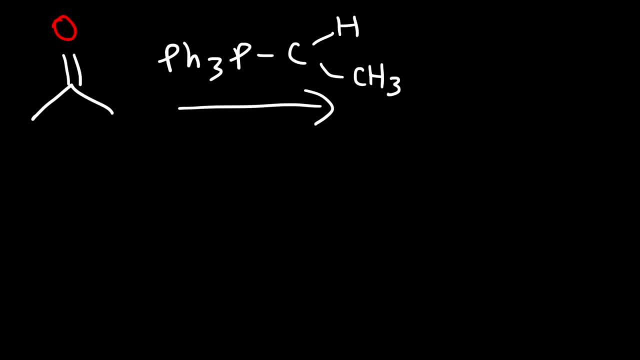 So we're going to have a hydrogen and a methyl group on this carbon, And so in this form, the phosphorus has a positive formal charge And the carbon has a negative formal charge. So how can we draw the product if the illid is given to us like this? 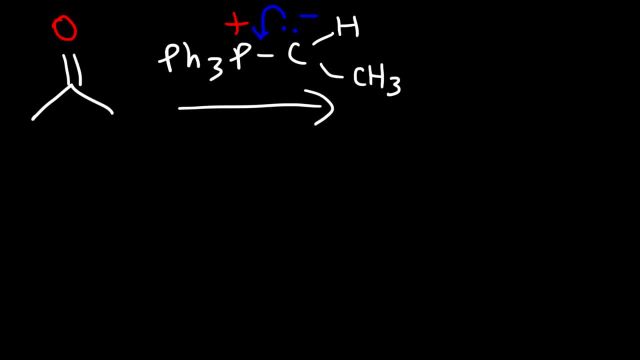 So we're going to do that. What I would do is draw the resonance form of this illid, And so it looks like this: The next thing I would do is basically rotate this ketone such that the double bond O is facing this double bond. 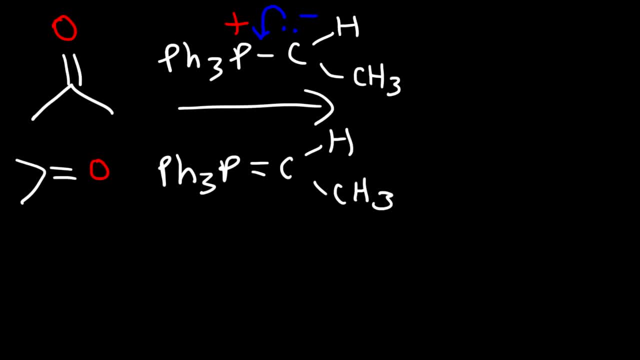 And then the next thing I'm going to do is replace the oxygen with this group, And so the product of this reaction is going to look like this. Now let's say we have this particular reactant, acetaldehyde, And let's react it with an illid that looks like this: 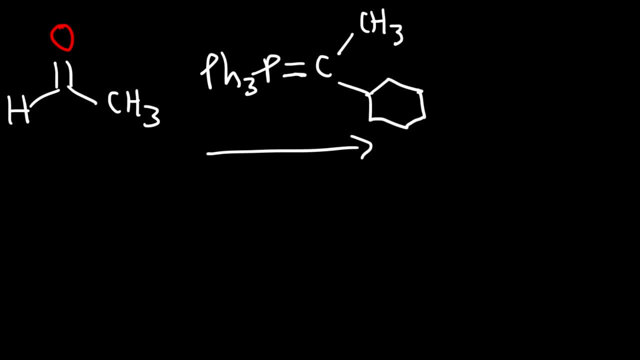 So draw the products of this reaction. So the first thing I would do is basically change the orientation of this molecule, And so I'm going to write it like this, And then all we need to do is replace the oxygen of the carbonyl group with what we see here. 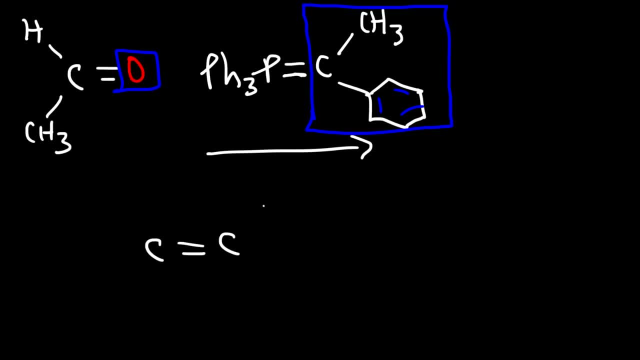 And so we can get this alkene where the two methyl groups are trans to each other. Now we can also get another type of alkene, For instance, if we replace the CH3 with the hydrogen. if we switch them, we get this. 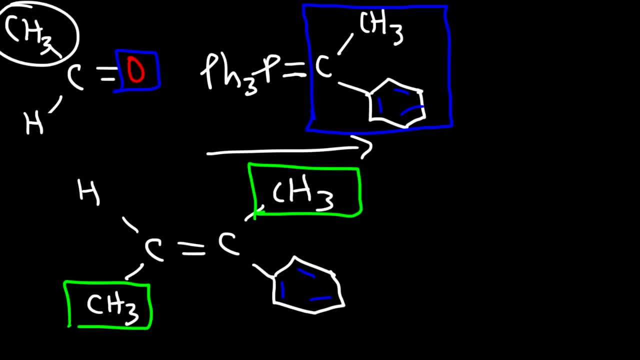 Then the two CH3s could be on the same side, And so we can get the other isomer, And so you can get a mixture of isomers for the Wittig reaction, And so this is the other product. Now let's go over the mechanism of the Wittig reaction. 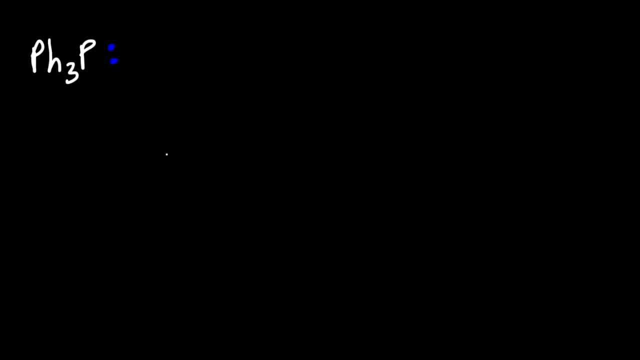 So the first thing that's going to happen is we're going to have triphosphate, So we're going to have triphenylphosphine And it's going to react with an alkyl halide in an SN2 reaction. So, because this is an SN2 reaction, primary alkyl halides will work very well. 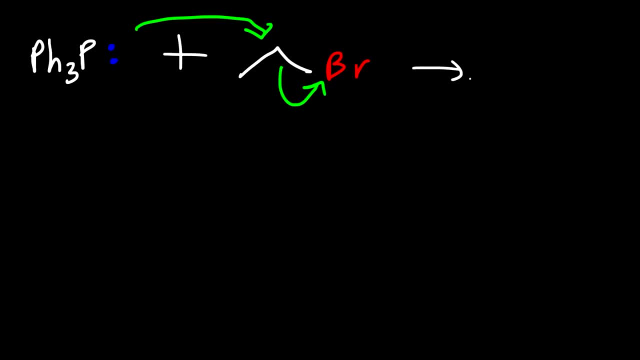 Tertiary alkyl halides will not work. Secondary is like: hmm, you got to be careful with those, But ideally you want to use a primary alkyl halide, And so what's going to happen is the phosphorus atom is going to be attached to this carbon. 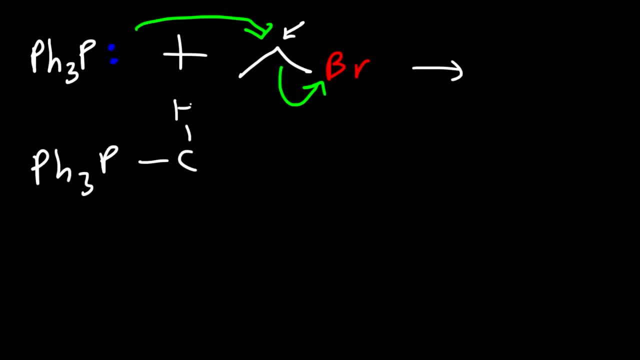 And that's going to be the carbon that's going to be attached to this carbon, And that's going to be the carbon that's going to be attached to this carbon, So that carbon has two hydrogens right now And it also has a CH3 group. 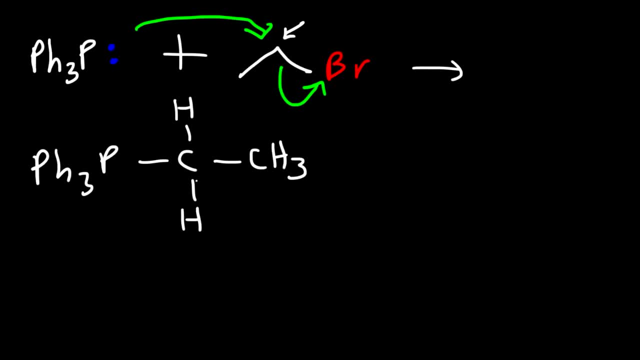 Now, whenever phosphorus, like nitrogen, has four bonds, it's going to have a positive formal charge. Now, in the next step, what we need to do is react this with butyl lithium. Whenever a carbon is bonded to a metal, that carbon is nucleophilic. 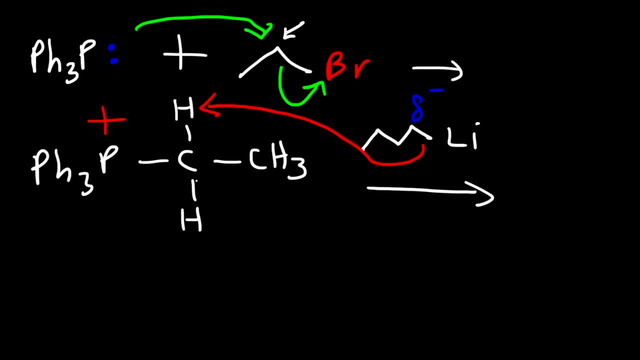 And it's a strong base. So what it's going to do is it's going to take off the hydrogen, put in a negative charge on this carbon, And so we have a resonance form of the illid. And so here's the other resonance form. 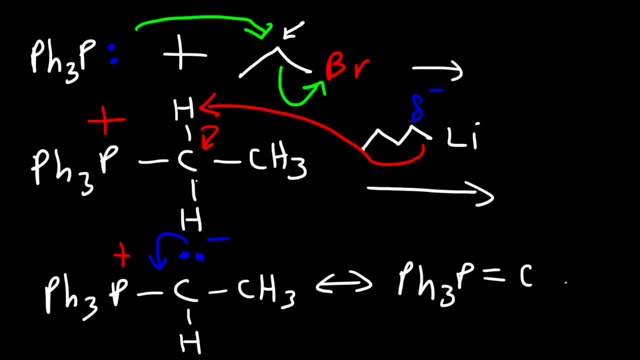 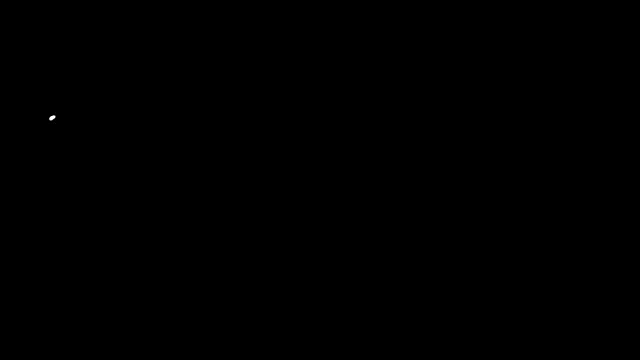 So you can write it in any one of these two ways. So now let's see how the illid is going to react with a ketone. So I'm going to use this form of the illid where the carbon has a negative formal charge. 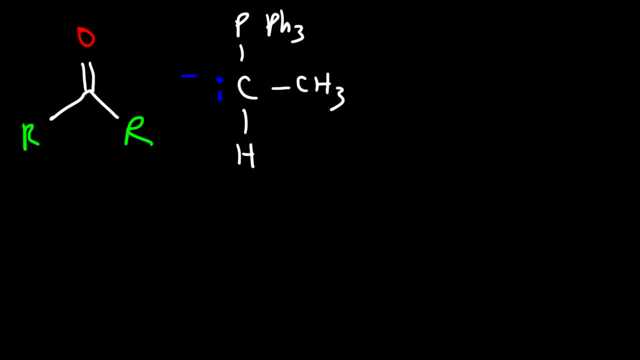 Now you want to set it up like this, because the nucleophilic carbon with the negative formal charge is going to react with a ketone, So the nucleophilic carbon with the negative formal charge is attracted to the partially positive carbonyl carbon. 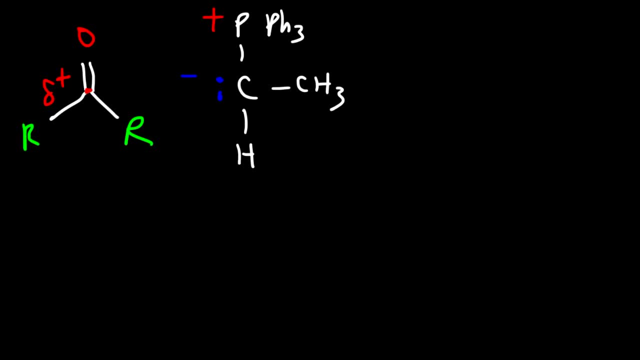 And the phosphorus, which has a positive formal charge, is attracted to the oxygen with its negative partial charge. So the nucleophilic carbon will attack the carbonyl carbon, causing the pi bonds to break, And those pi electrons will be used to connect the oxygen and the phosphorus together. 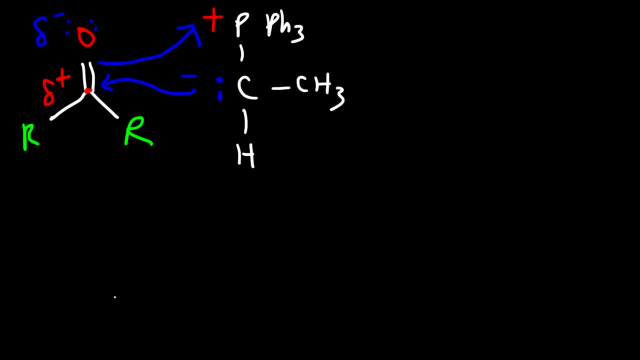 And so you're going to get this four-membered ring That looks like this. So I'm going to draw this carbon atom. So we have a carbon and another carbon and a single bond between a carbon and the oxygen, And now the oxygen is attached to the phosphorus group. 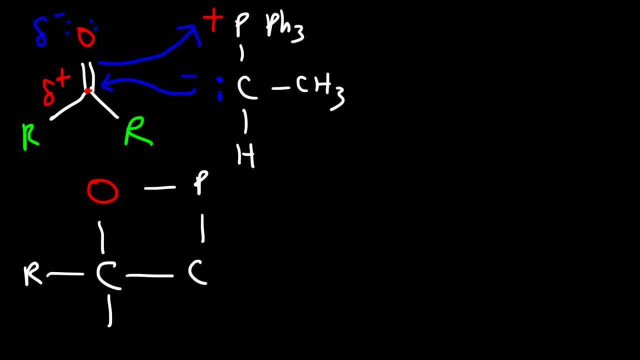 And so here's the two R groups of the electrophilic carbon, And here's the hydrogen and the methyl of the nucleophilic carbon, And here's the three, And here's the three phenyl groups. Now these two bonds will break. 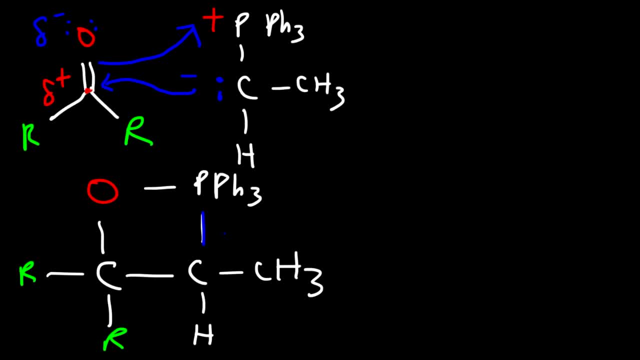 So let's talk about this bond first, the bond between the carbon and the phosphorus atom. Which of these two atoms is more electronegative, carbon or phosphorus? It turns out that carbon is more electronegative than phosphorus. 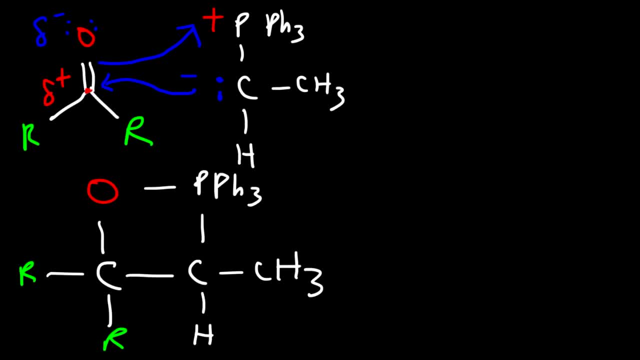 And you can look this up online. If you type in electronegativity table in Google Images, you can verify that. So, because carbon is more electronegative, when this bond breaks, carbon is going to pull those electrons toward itself. 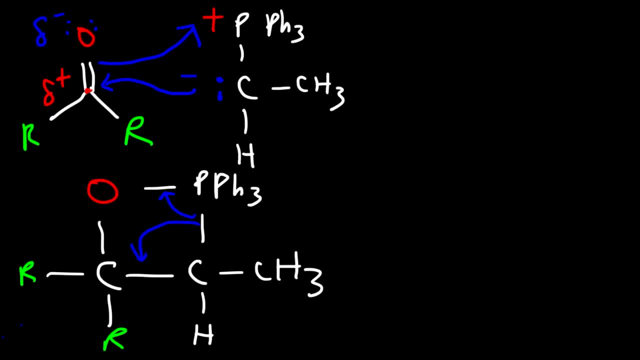 So those electrons will go here as opposed to going here, So they're going to go towards the more electronegative carbon. Likewise, when this bond breaks, those electrons are going to go towards the more electronegative oxygen atom, Because oxygen is more electronegative than carbon. 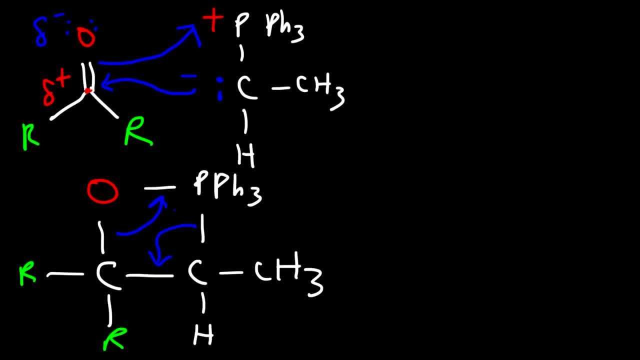 And so whenever a bond breaks, those electrons, Electrons will tend to go towards the more electronegative atom, And so at this point, when this oxophosphatine group breaks apart, we're going to get an alkene. 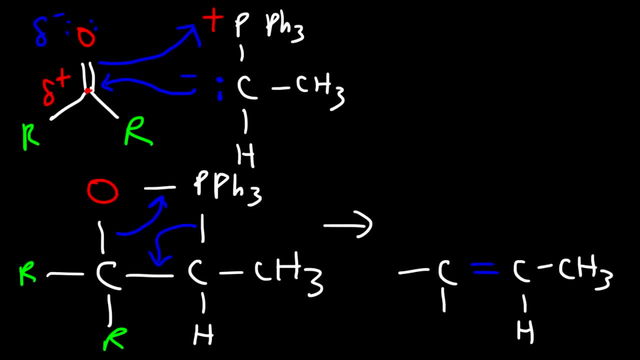 Which in this case looks like this, And the other side product will be triphenylphosphene oxide, And so that's the mechanism for the Wittig reaction. And so that's it. Now let's talk about the Bayer-Villager oxidation reaction. 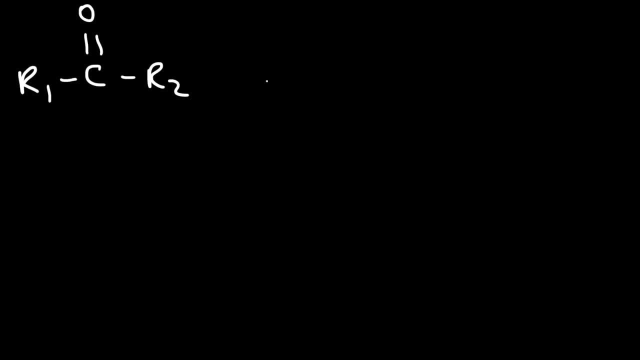 And so we're going to react a ketone with a peroxyacid, And in order to draw the product of this reaction, all we need to do is insert an oxygen, either between R1 and the carbonyl carbon or between R2 and the carbonyl carbon. 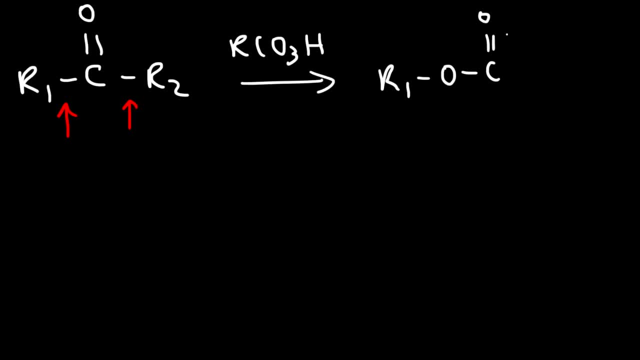 So the product could look like this, Or it can be like this: The side product is a carbosilic acid, So basically, an oxygen is transferred from the peroxyacid to the ketone, turning it into an ester. 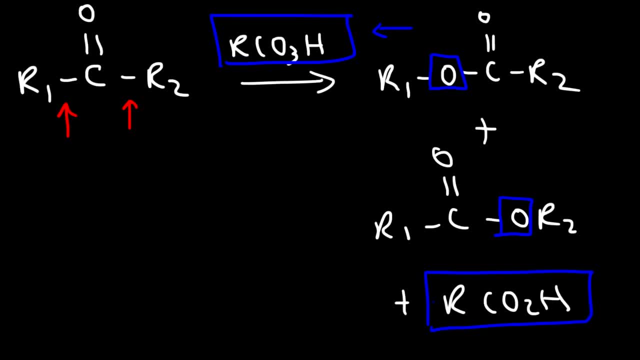 And so the peroxyacid becomes a carbosilic acid as it loses an oxygen atom. Now how can we determine which R group is going to have the oxygen? Is it going to be R1 or R2? So we need to determine which R group has a greater migratory aptitude. 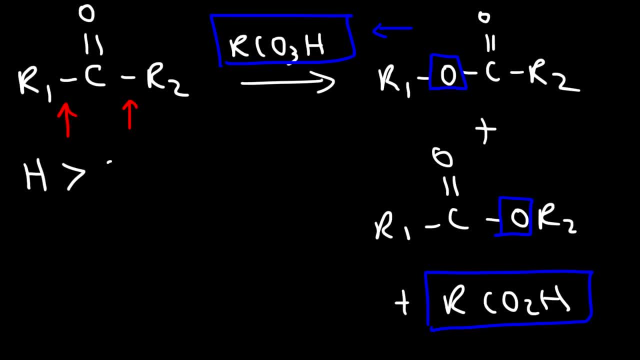 And it turns out that hydrogen has a greater migratory aptitude than a tertiary alcohol- I mean not alcohol but tertiary alkyl group- And that's higher than a secondary alkyl group which has the same migratory aptitude as a phenyl group. And that's better than a primary alkyl group, which is better than a methyl group. And so let's go over some examples. Let's start with acetaldehyde. So what is the major product of this reaction? So let's write both possibilities. 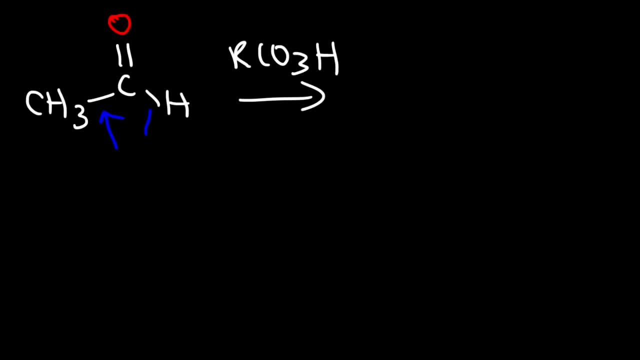 We can insert the oxygen between the carbon and the methyl group or between the carbonyl carbon and the hydrogen group. So this is one possibility And here is the other possibility. So which of these two answers is the major product? Hydrogen has a greater migratory aptitude than the methyl group. 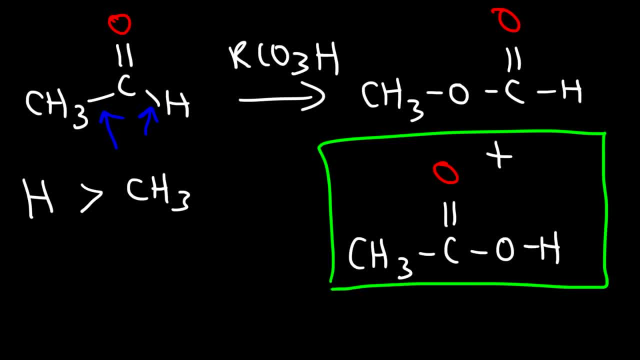 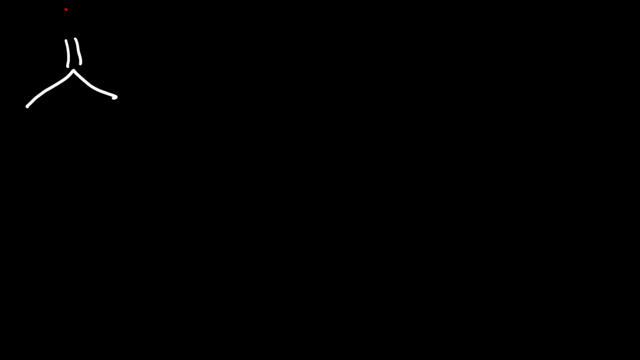 So therefore, this is going to be the major product. So whenever you use a peroxy acid on an aldehyde, it's going to be oxidized to a carbosilic acid. Now let's work on some practice problems. Go ahead and react propanone with a peroxy acid. 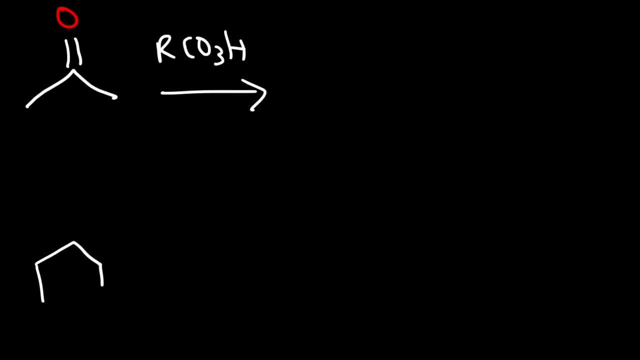 and produce a peroxy acid. Now we're going to predict the major product. Also, we're going to use cyclopentanone as well, So go ahead and try these reactions Now. both of these ketones are symmetrical, and so it really doesn't matter where we put the oxygen atom. 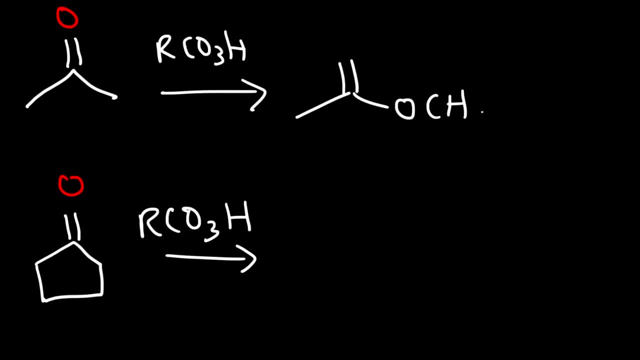 So I'm just going to put it on the right side. Therefore, the Bayer-Villager oxidation reaction is very useful for converting oxygen atoms. So I'm just going to put it on the right side. Therefore, the Bayer-Villager oxidation reaction is very useful for converting oxygen atoms. 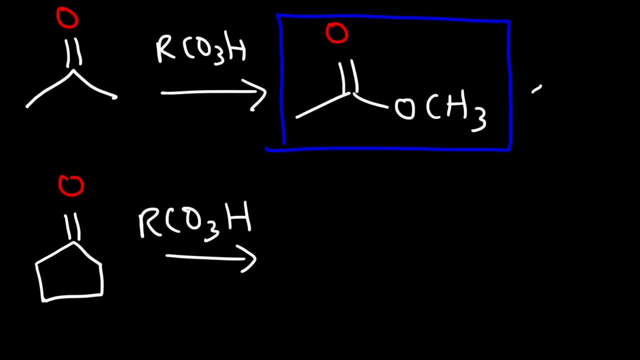 So I'm just going to put it on the right side. Therefore, the Bayer-Villager oxidation reaction is very useful for converting oxygen atoms. Now, in the case of a cyclic ketone, we're going to get a lactone, So we started with a five-membered ring. 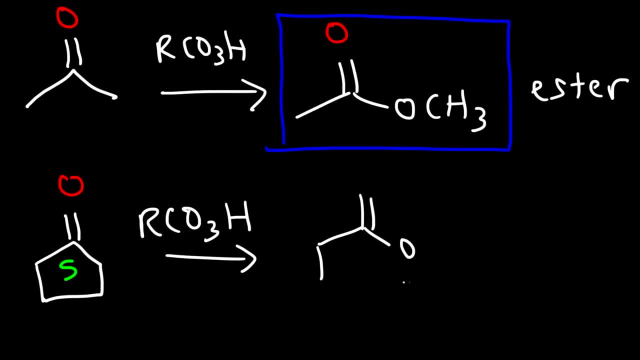 Now we're going to introduce the oxygen to this ring, So it's going to be a six-membered ring. So this is called a lactone, So it's a six-membered ring. Now we're going to introduce the oxygen to this ring. 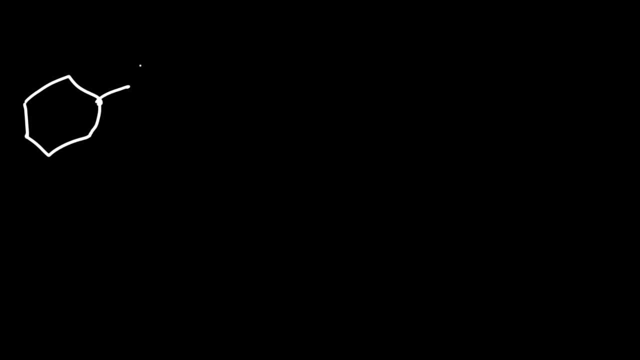 So it's going to be a six-membered ring. So here is another example. What is the major product of this reaction? So let's draw both possibilities. We can put the oxygen atom on the left side, Or we can put it on the right side. 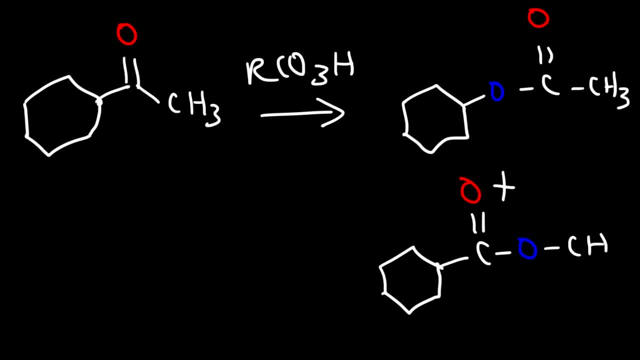 So which of these two products is the correct one? Should we put it on the left Or should we put it on the right? So we're comparing a secondary alkyl group. Even though this is a tertiary carbon, when you disconnect it, it's considered a secondary alkyl group because you no longer count on this carbon. 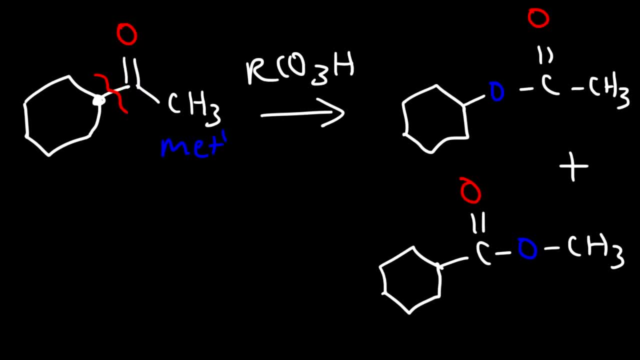 So we have a methyl group versus a secondary alkyl group. Now, based on what I gave you earlier, we know that hydrogen is the best. Then it's the tertiary alkyl group And then the secondary alkyl group, which is about the same as the phenyl group. 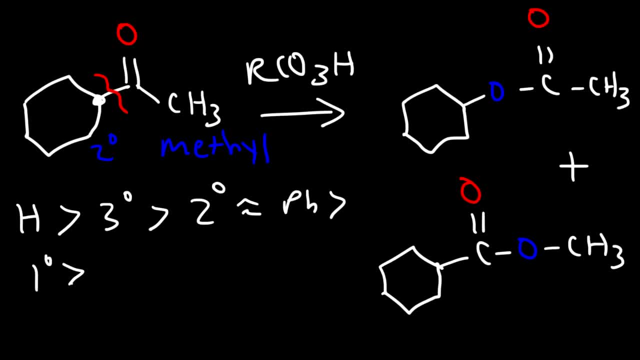 And then it's the primary alkyl group And then the least reactive is the methyl group. So it's definitely not going to be the methyl group. Therefore, we're going to put the oxygen atom with the secondary alkyl group. So this is the answer. 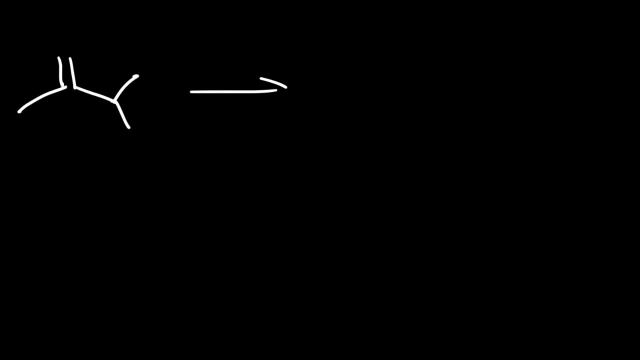 Now let's do one last example. So go ahead and produce a reaction. Take the major product of this reaction. So we have a methyl group on the left and an isopropyl group on the right. Well, we know, the methyl group has the least migratory aptitude. 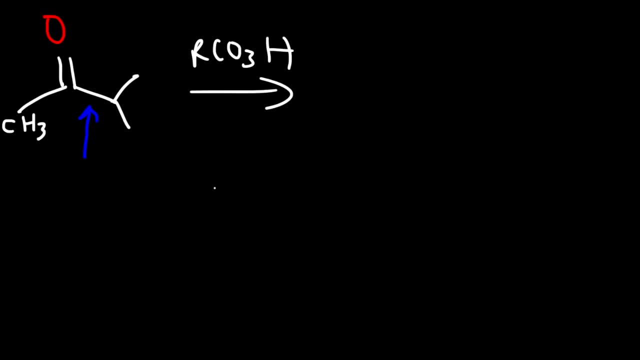 So, therefore, we need to put the oxygen between the carbonyl carbon and the isopropyl group. And so now you know how to find the major product of the Bayer-Villager oxidation reaction. And, as you can see, it converts ketones into esters. 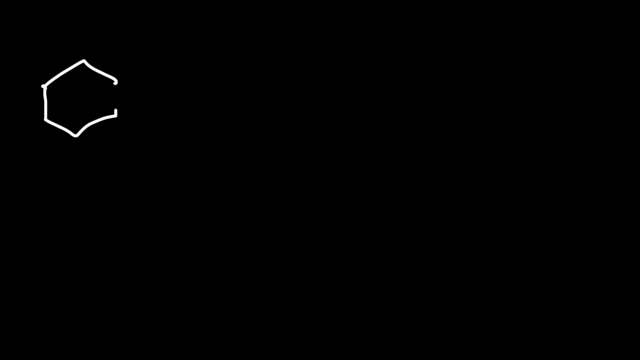 Now there's one more topic that we need to talk about, And it is the direct addition reaction versus the conjugate addition reaction, And so here we have an alpha-beta unsaturated ketone. As you can see, there's a double bond between the alpha and beta carbons. 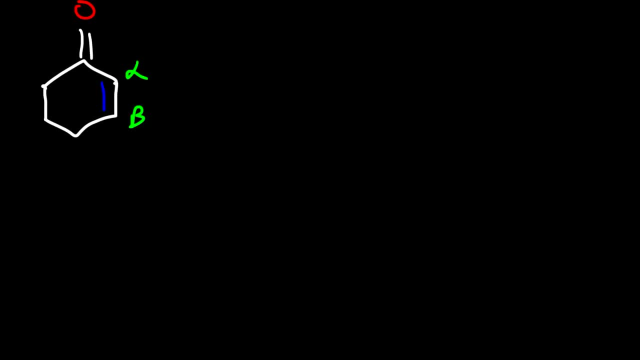 The alpha carbon is one carbon away from the carbonyl group. The beta carbon is two carbons away from the carbonyl group, And alkenes are unsaturated because they have less hydrogen atoms than alkenes do. Alkenes are fully saturated with hydrogen atoms. 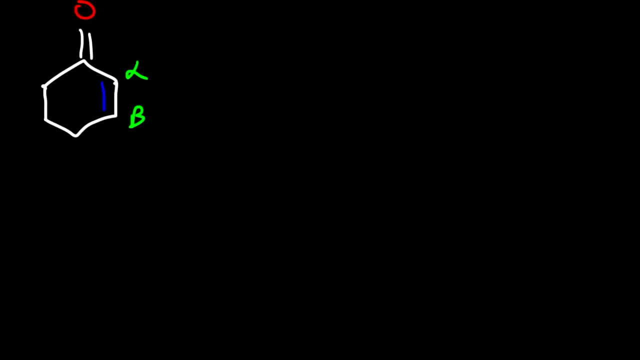 Alkenes. they're deficient in hydrogen atoms compared to alkenes, So we have an alpha-beta unsaturated carbonyl compound. Now it's important to understand that: the beta carbon and the carbonyl carbon. they're electrophilic. 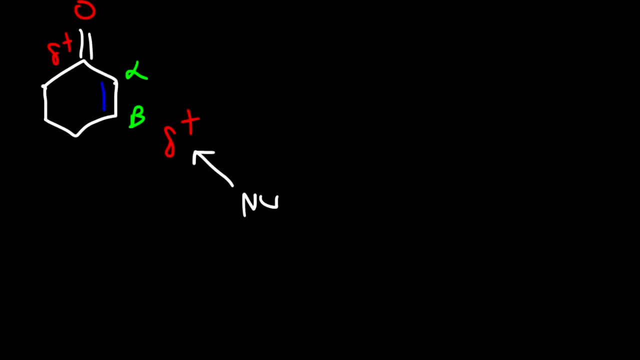 The nucleophile can attack at the beta carbon or it can attack at the carbonyl carbon. If it attacks at the beta carbon, we have conjugate addition, And if it attacks at the carbonyl carbon, it's known as direct addition. 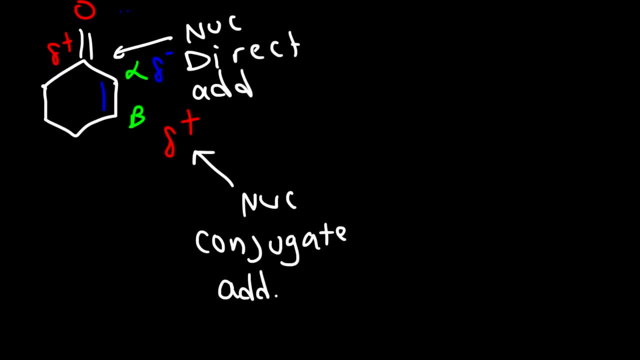 Now, the alpha carbon is nucleophilic And so is the oxygen, So you can show this using resonance structures. So we could take this double bond, move it here and break the pi bond. If we do so, we're going to have a negative charge on the oxygen atom. 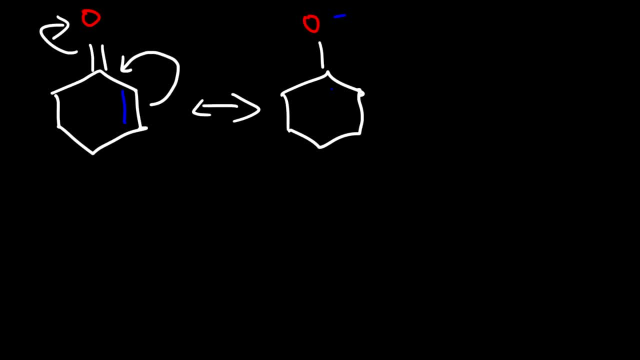 And there's a double bond here and there's a positive charge on the beta carbon, And so thus you can see that the beta carbon is electrophilic due to the positive formal charge and the oxygen atom is nucleophilic due to the negative charge on it. 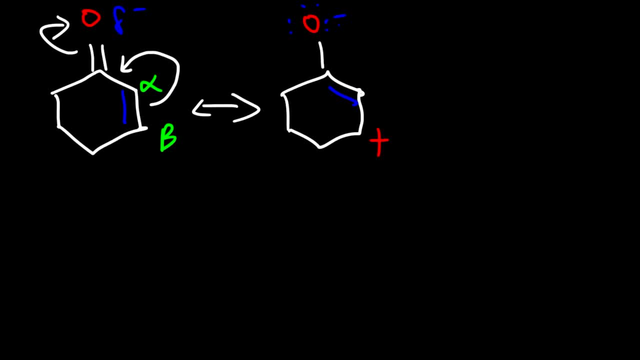 Now we can draw another resonance structure if we take a lone pair, form a pi bond and push these electrons on this carbon, And so we can draw another resonance structure. And so we can draw another resonance structure if we take a lone pair, form a pi bond and push these electrons on this carbon. And so we can draw another resonance structure if we take a lone pair, form a pi bond and push these electrons on this carbon. And so we can draw another resonance structure if we take a lone pair, form a pi bond and push these electrons on this carbon. 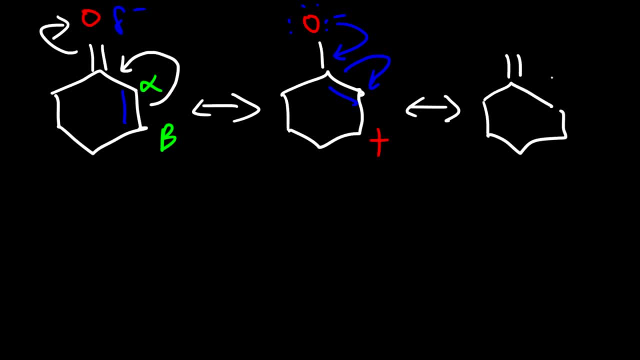 And so this shows that the alpha carbon is nucleophilic since it has a negative formal charge. Now, starting from the original alpha-beta unsaturated compound, we can also draw this. We can draw another resonance structure if we take a lone pair, form a pi bond and push these electrons on this carbon. 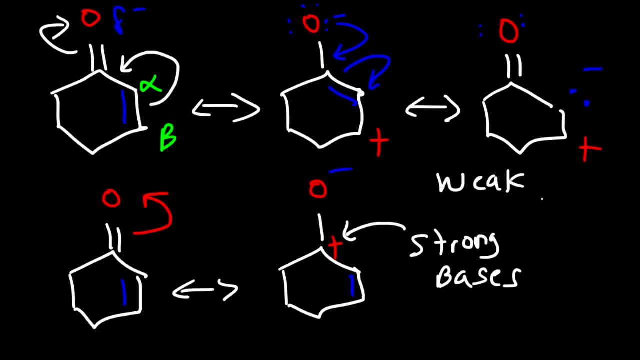 And so this shows that the theta carbon is nucleophilic. since it is nucleophilic, And so this shows that the theta carbon is nucleophilic, and since it has a negative formal charge on it, weak bases- they prefer to attack the beta-carbon, And so weak bases they. 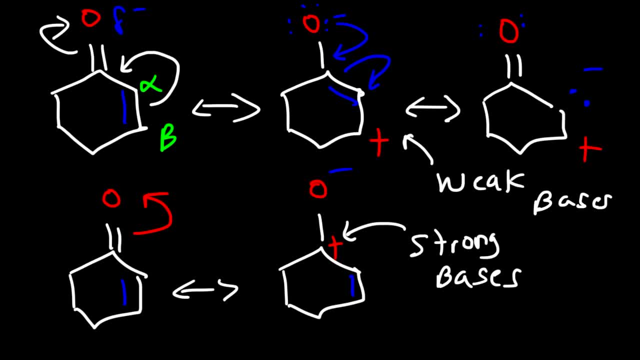 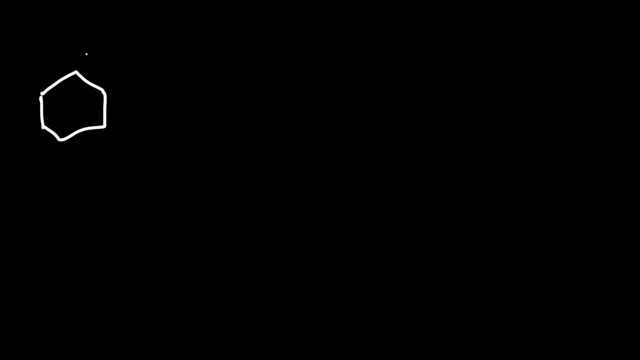 favor conjugate addition, whereas a strong base favors direct addition. Now let's go over some examples. Let's use the Grignard reagent. The Grignard reagent is a very strong base, and so it's going to favor direct addition. So therefore, it's going to go. 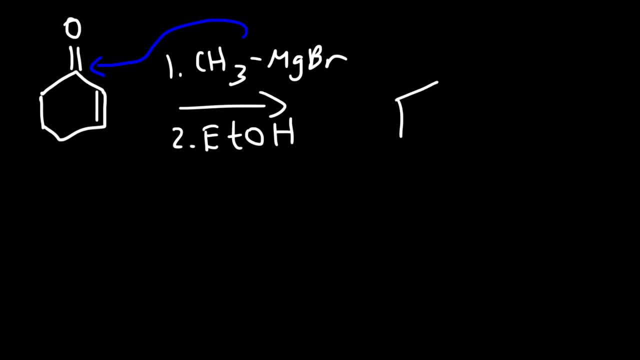 to the carbonyl carbon, And so the final product will look like this: We're going to get an OH group and we're going to add the methyl group to the carbonyl carbon, And so the double bond will be unaffected. Now let's use a weak base. 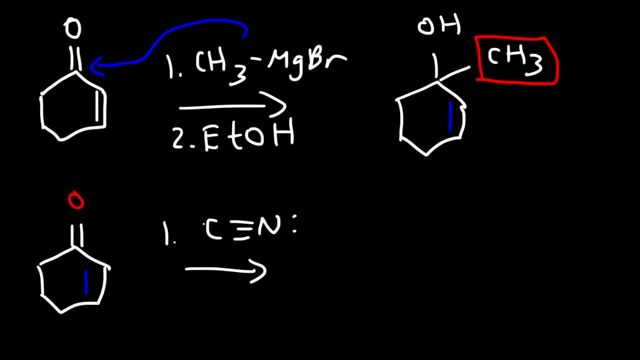 A good example is the cyanide ion. It's a good nucleophile, but it's a weak base, And so weak bases tend to go for the beta-carbon, and so they favor conjugate addition. So the cyanide group will be here. So this is conjugate addition, and above we 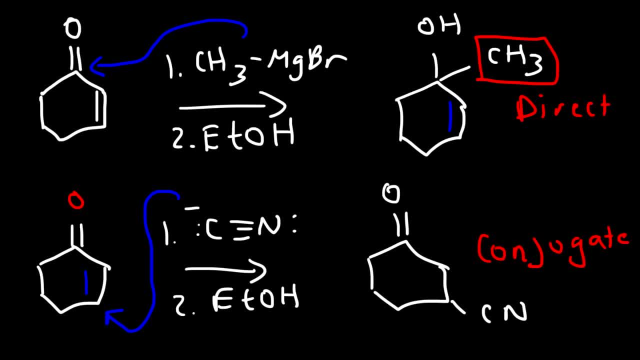 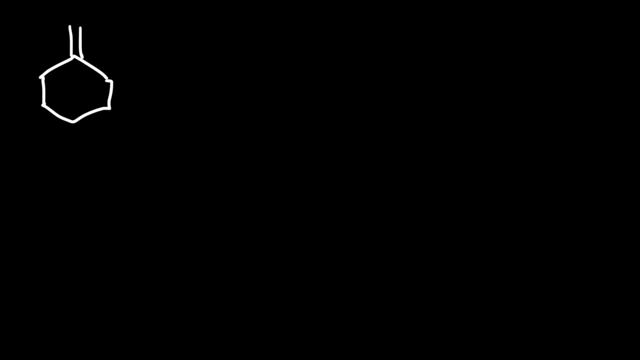 have direct addition. So keep in mind: strong bases, they favor direct addition and weak bases favor conjugate addition. Here's another example. So what about the Gilman reagent? So let's say we have this organocopper lithium reagent, Is it considered a? 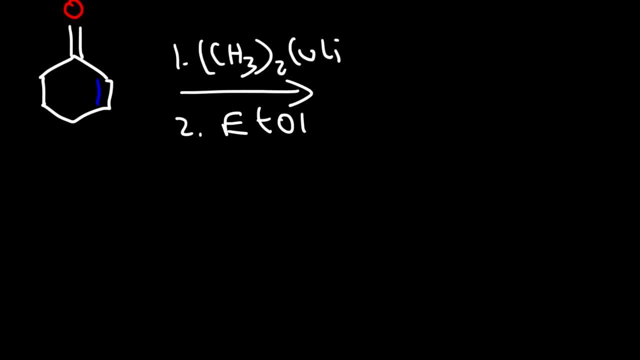 strong base or weak base. With the Gilman reagent it's going to go for the beta-carbon, So it's not as strong as the Grignard reagent. Therefore, we're going to get this product. So that's how we can put a methyl group on the beta-carbon. 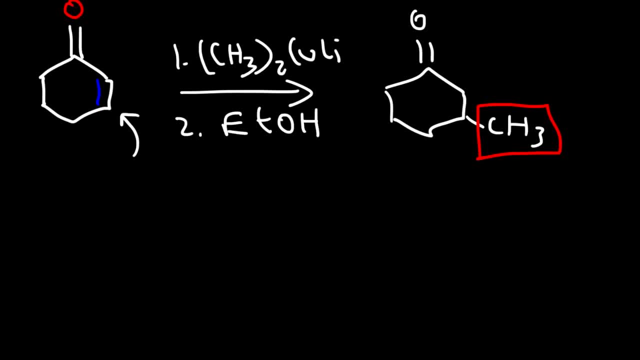 using the Gilman reagent. Here's another example. Let's say, if we use sodium borohydride with this molecule, This reagent can produce a mixture of products for this specific type of ketone. So you can get direct addition by adding the hydrogen here and you can. 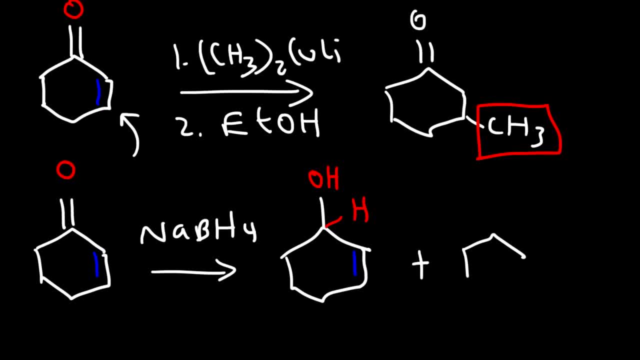 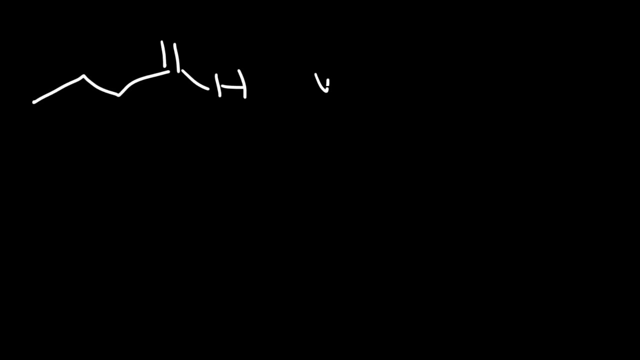 also get conjugate addition, with the hydrogen being added at that carbon, And so that reaction gives you a mixture of products. Consider these two compounds, a conjugated ketone and a conjugated carbon aldehyde: which compound favors direct addition and which one favors conjugate? 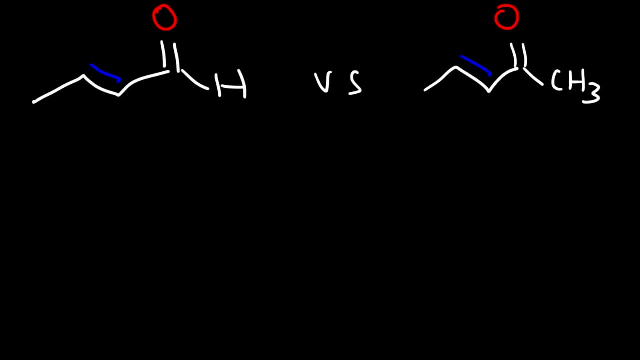 addition. now the one that favors direct addition is the one that's most accessible, and for the aldehyde, the carbonyl part of the molecule is more accessible towards a direct addition. in the case of the ketone, the methyl group creates steric hindrance, so it's harder for the nucleophile to approach the carbonyl compound, therefore aldehydes, they favor direct addition. aldehydes are more electrophilic than ketones. the methyl group is an electron donating group, and so it donates electron density to the carbonyl functional group, making it less electrophilic, and so ketones they 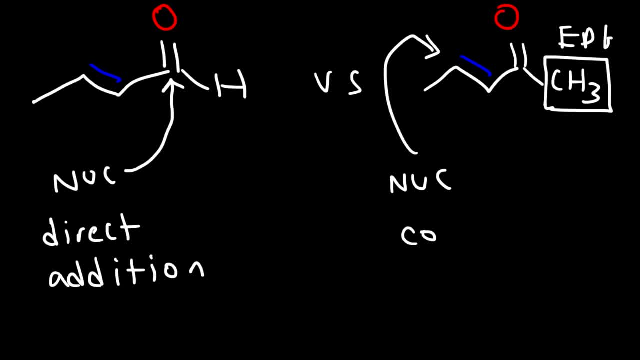 favor conjugate addition, whereas aldehydes, which are more accessible, favor direct addition. so even if you have, let's say, a greenery agent which favors direct addition, if, if the ketone is sterically hindrance, the greenery agent which favors direct addition may have no choice but to. 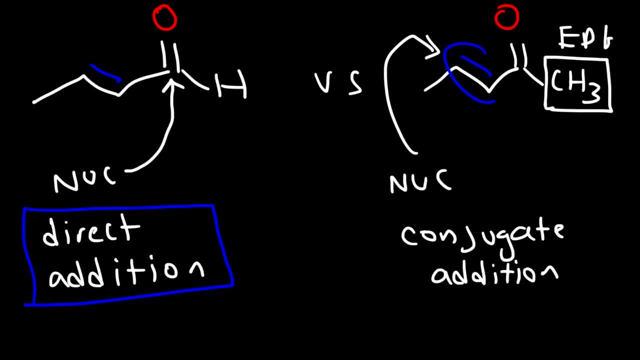 attack at the beta carbon given the conjugate addition product. so even with greenery agents you can increase the yield of the conjugate addition product by making the carbonyl part of the molecule less accessible. so you need to consider two factors: the strength of the base and any steric hindrance so strong? 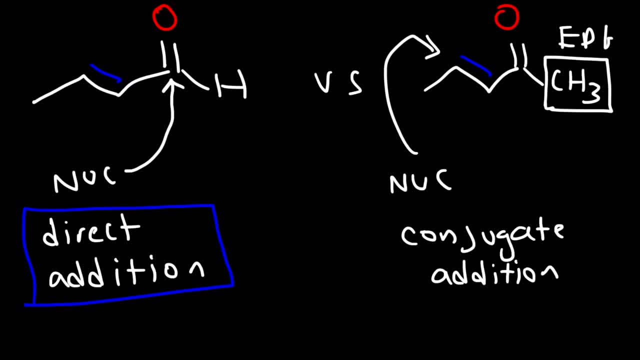 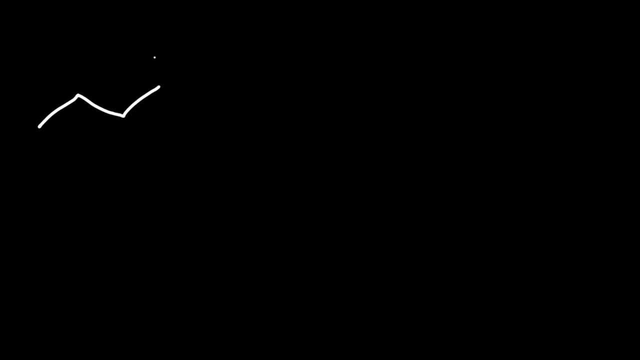 bases like a greenery agent, they favor direct addition. weak bases favor conjugate addition. ketones: they favor conjugate addition and aldehydes favor direct addition. so let me give you an example problem. so here we have two ketones. so looking at the key tone on the left, that key tone does it favor direct. 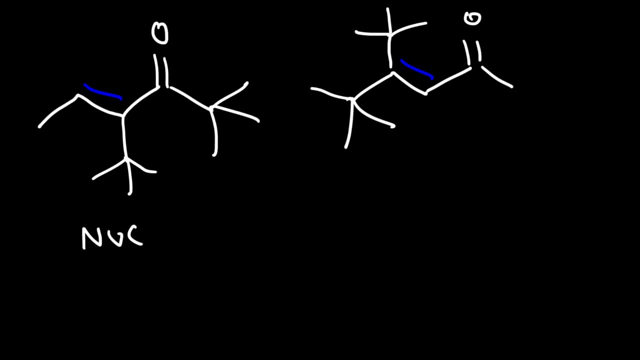 addition or conjugate addition. now, this nucleophile is going to have a hard time accessing this carbonyl group and so it's not going to go there. but notice that the beta carbon is more accessible. so this particular key tone, it's going to favor conjugate addition over direct addition. 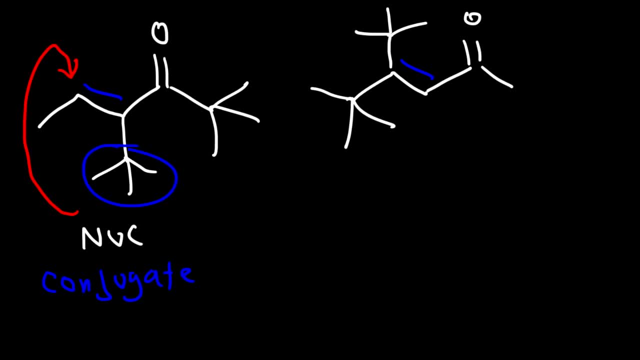 because the nucleophile it can't get past these to butyl groups to basically do direct addition. so the carbonyl group is inaccessible. therefore the nucleophile is going to favor conjugate addition. so ketones may perform conjugate addition in addition to direct addition. now looking at this, 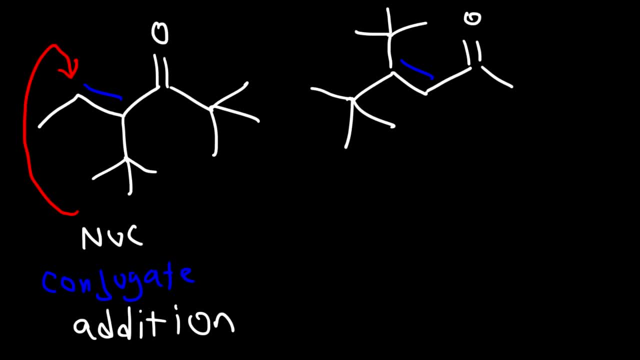 example here, notice that the beta carbon is blocked by these to butyl groups, so it's inaccessible. therefore, the nucleophile has the easier time attacking the carbonyl group, and so it's going to favor direct addition over conjugate addition, and so you need to consider steric factors as well as the strength of the 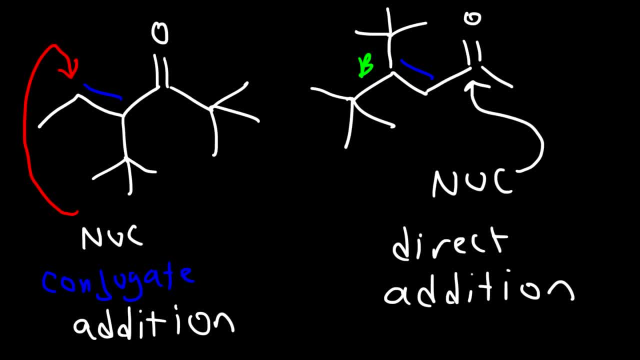 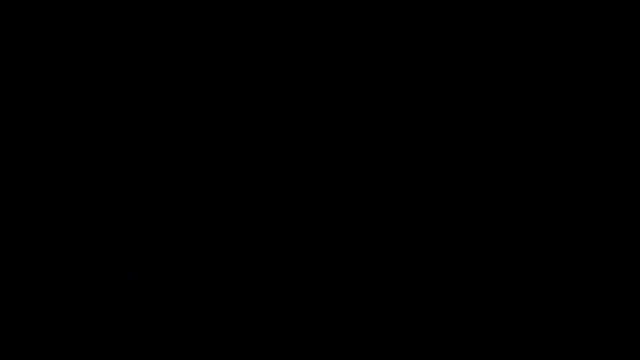 base to see which of these two pathways will lead to the major product. so now let's go over the mechanism of direct addition reaction. so the first thing we're going to do is react it with a strong base. Now, in this case, both the beta carbon and the carbonyl carbon. they're relatively 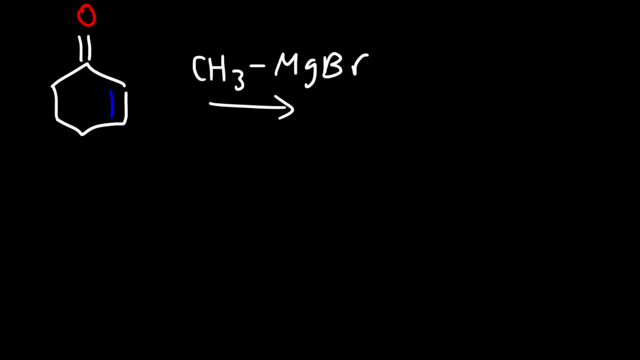 accessible to the green reagent. So the strength of the base will determine which one is going to lead to the major product. So because we have a strong base and none of these carbons are sterically hindered, then the green reagent is going to attack the carbonyl carbon. 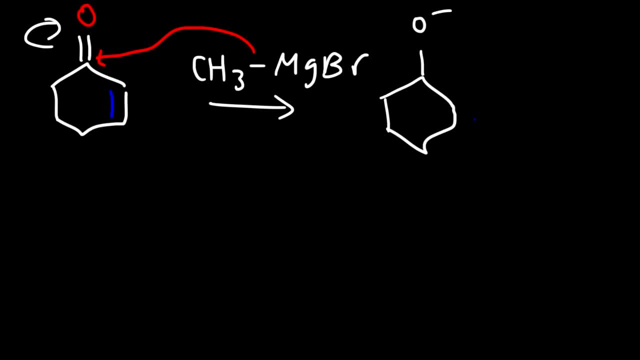 And so we're going to get an oxygen with a negative charge, and then, in the next step, we can use the solvent, which could be ethanol or something else, to protonate the oxygen, And so that's the mechanism for the direct addition reaction. 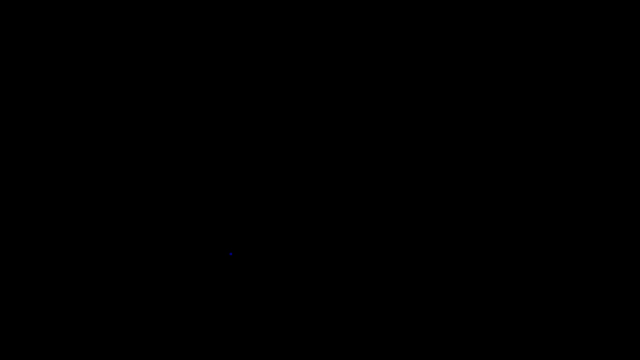 Now let's go over the mechanism for the conjugate addition reaction. So in this case I'm going to use cyanide. So cyanide is going to attack the beta carbon because it's a weak base. The pi bond will break, And so we're going to get an oxygen. 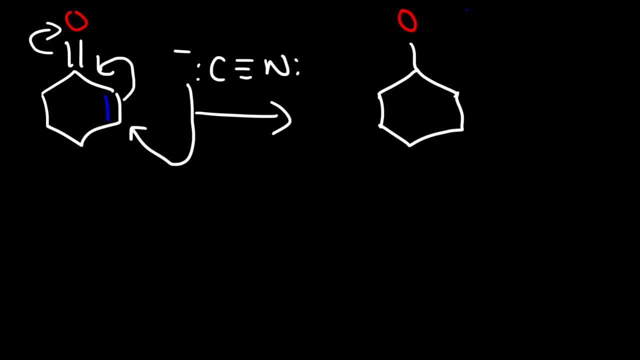 atom with a negative charge And we have a double bond between the carbonyl carbon and the alpha carbon. And here is the Cn group. Now, in the next step, we'll need to add a hydrogen to the alpha carbon. Keep in mind, the alpha carbon is nucleophilic, So when the oxygen with a